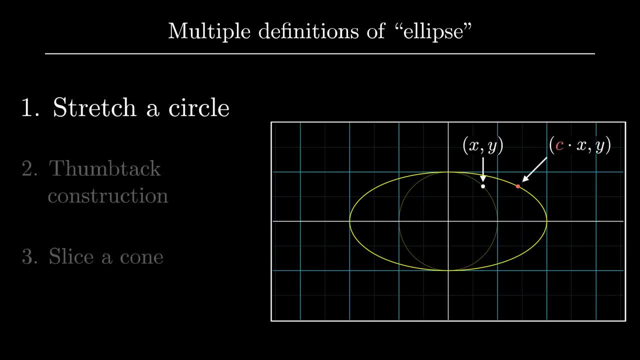 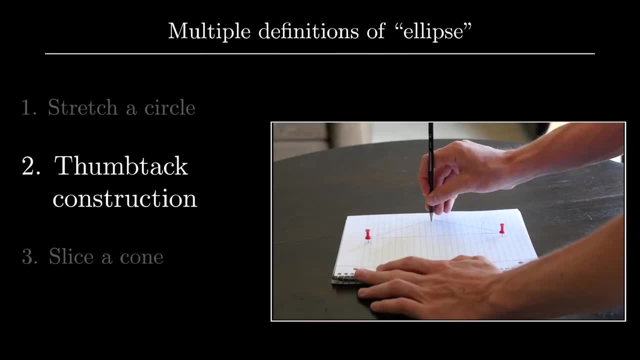 the x coordinate by some special factor for all the points. Another is the classic two thumbtacks and a piece of string construction where you loop a string around two thumbtacks stuck into a piece of paper and pull it taut with a pencil and then trace around, keeping the string taut the whole. 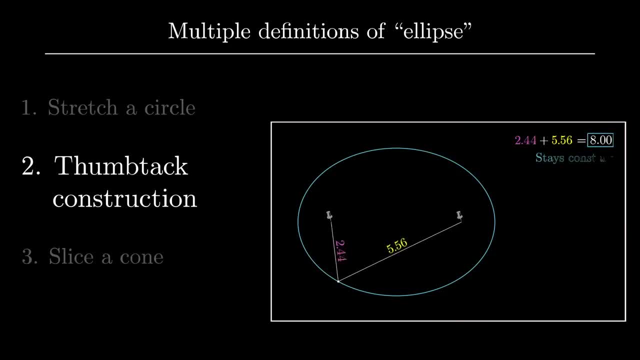 time. What you're drawing by doing this is the set of all points, so that the sum of the distances from each pencil point to the center of the circle is equal to the sum of all points. So the sum of the to the two thumbtack points stays constant. 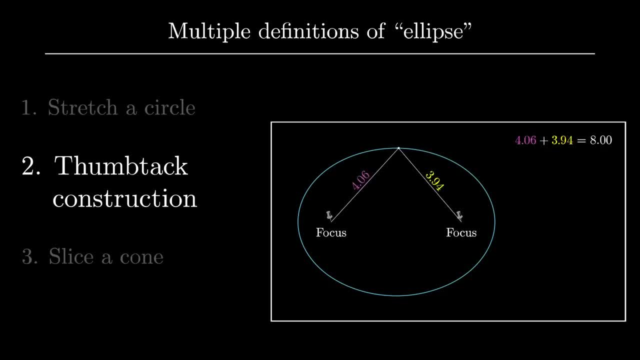 Those two thumbtack points are each called a focus of the ellipse, and what we're saying here is that this constant focal sum property can be used to define what an ellipse even is. And yet another way to define an ellipse is to slice a cone with a plane at an angle. 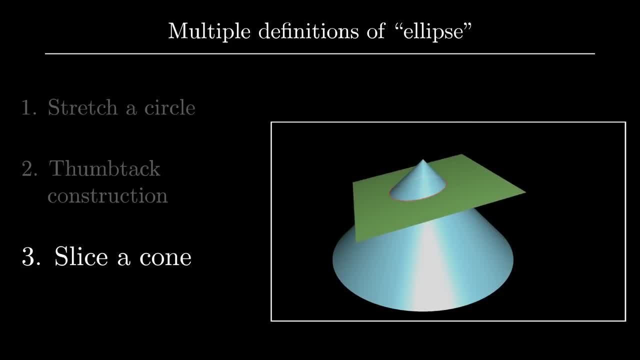 an angle that's smaller than the slope of the cone itself. The curve of points where this plane and the cone intersect forms an ellipse, which is why you'll often hear ellipses referred to as a conic section. Now, of course, an ellipse is not just one curve. it's a family of curves ranging from 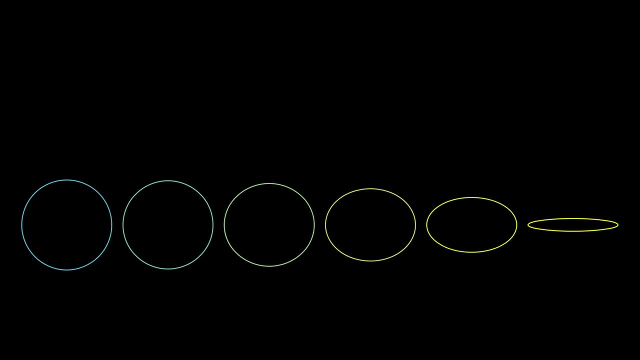 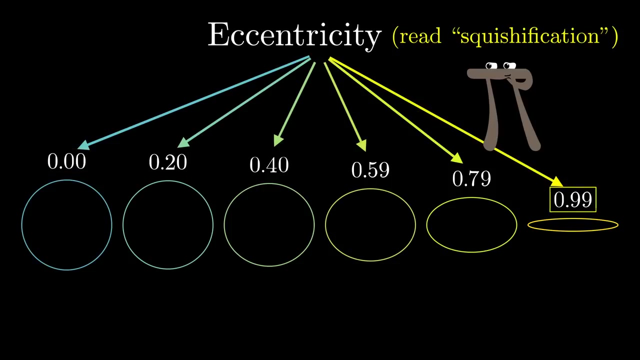 a perfect circle up to something that's infinitely stretched. The specific shape of an ellipse is typically quantified with a number called its eccentricity, which I sometimes just read in my head as squishification. A circle has eccentricity 0,, and the more squished the ellipse is, the closer its eccentricity. 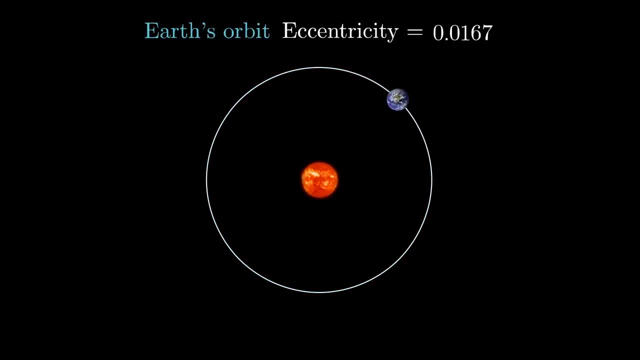 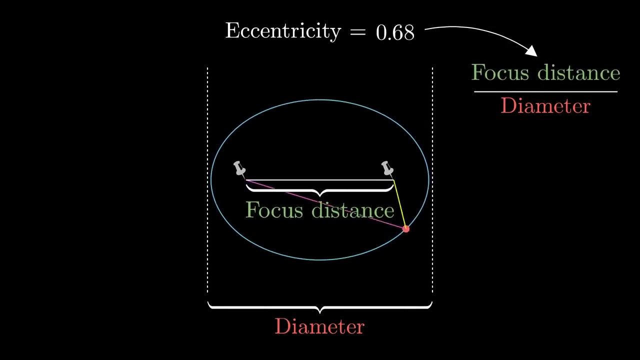 is to the number 1.. For example, Earth's orbit has an eccentricity of 0.. 0.. How its excentricity is determined by how far apart the two thumbtacks are, Specifically the distance between the two foci. 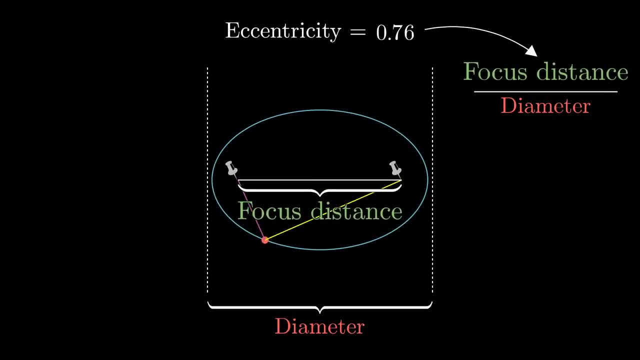 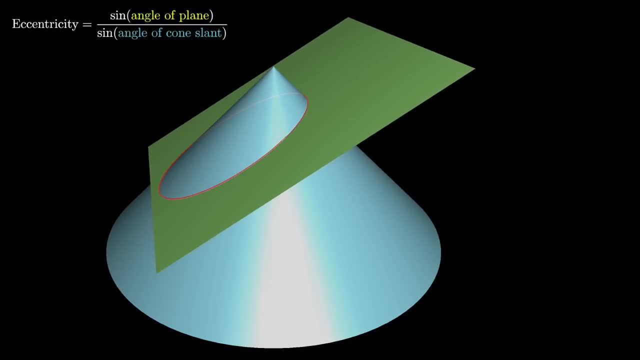 divided by the length of the longest axis of the ellipse For slicing a cone, the eccentricity is determined by the slope of the plane that you used for the slicing. And you might justifiably ask, especially if you're a certain Reddit user, why on earth? 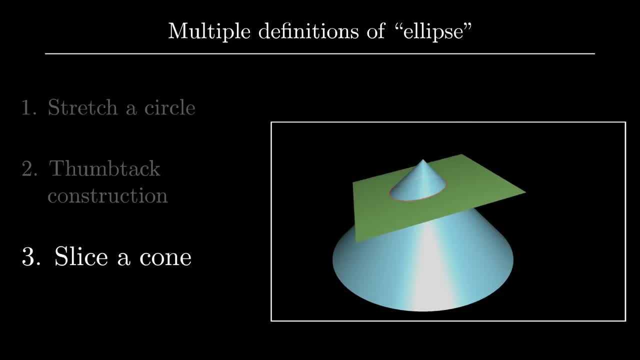 an angle that's smaller than the slope of the cone itself. The curve of points where this plane and the cone intersect forms an ellipse, which is why you'll often hear ellipses referred to as a conic section. Now, of course, an ellipse is not just one curve. it's a family of curves ranging from 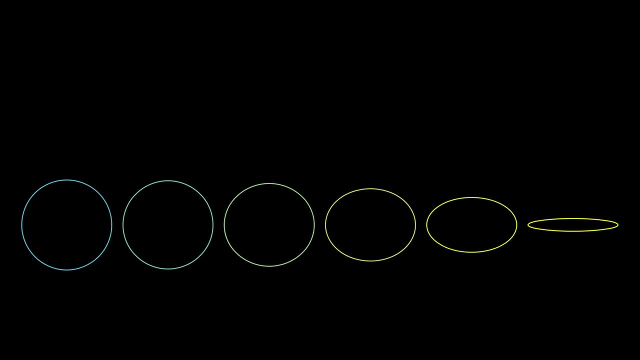 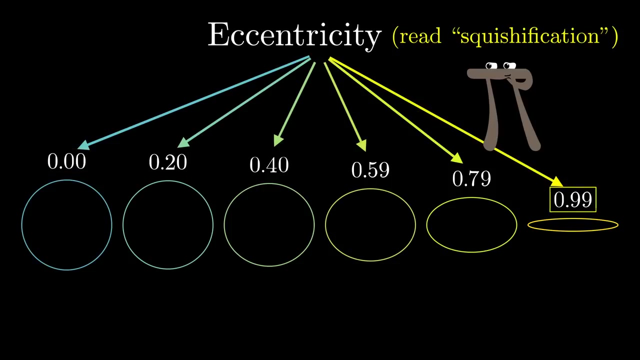 a perfect circle up to something that's infinitely stretched. The specific shape of an ellipse is typically quantified with a number called its eccentricity, which I sometimes just read in my head as squishification. A circle has eccentricity zero, and the more squished the ellipse is, the closer its eccentricity. 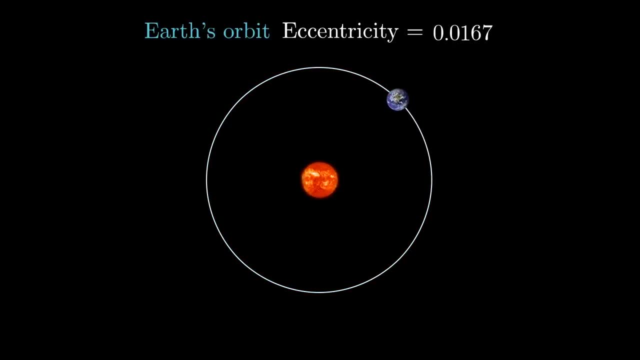 is to the number one. For example, Earth's orbit has a number one. Earth's orbit has an eccentricity 0.0167, very low squishification, meaning it's really close to just being a circle, While Halley's comet has an orbit with eccentricity 0.9671, very high squishification. 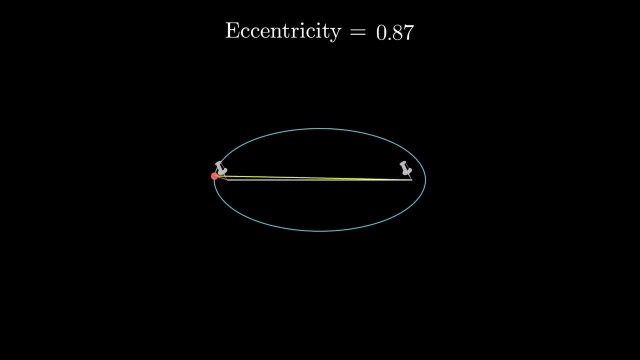 In the thumbtack definition of an ellipse based on the constant sum of distances from each point to the two foci. this eccentricity is determined by how far apart the two thumbtacks are. Specifically, it's the distance between the foci divided by the length of the ellipse. 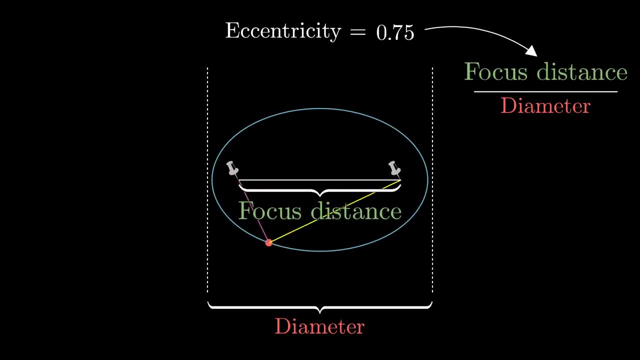 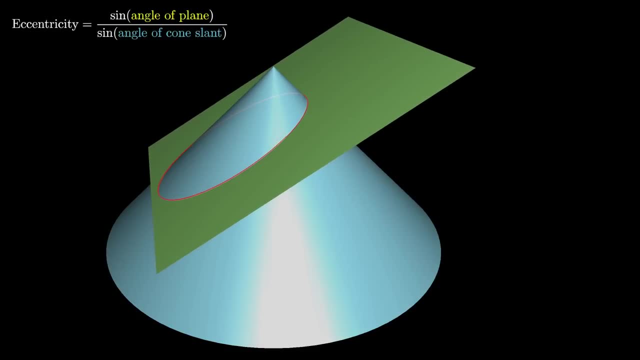 and divided by the length of the longest axis of the ellipse For slicing a cone, the eccentricity is determined by the slope of the plane that you used for the slicing. And you might justifiably ask, especially if you're a certain Reddit user, why on earth? 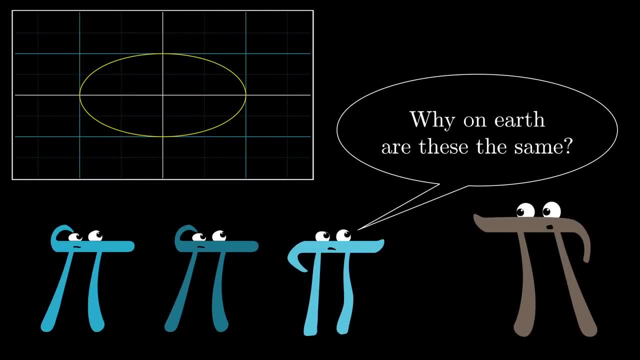 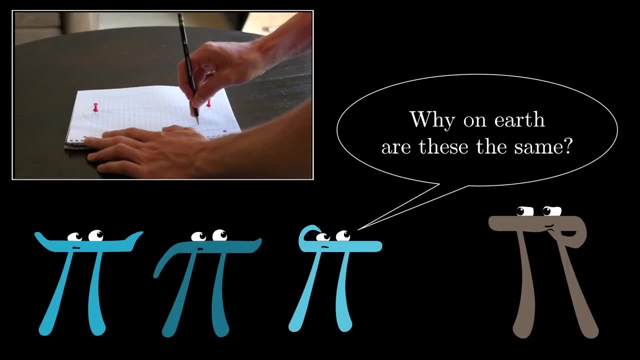 should these three definitions have anything to do with each other? I mean sure it kind of makes sense that each should produce some vaguely oval-looking stretched out loop, But why should the family of curves produced by these three totally different methods be precisely the same shapes? 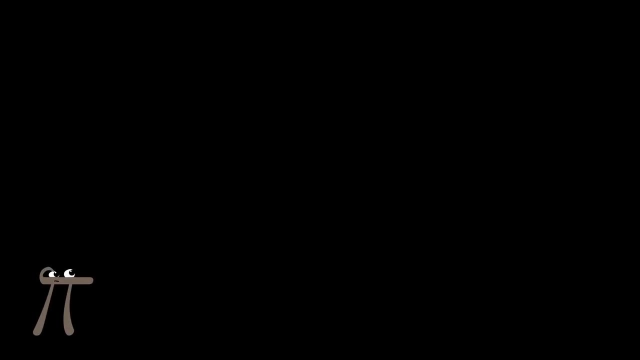 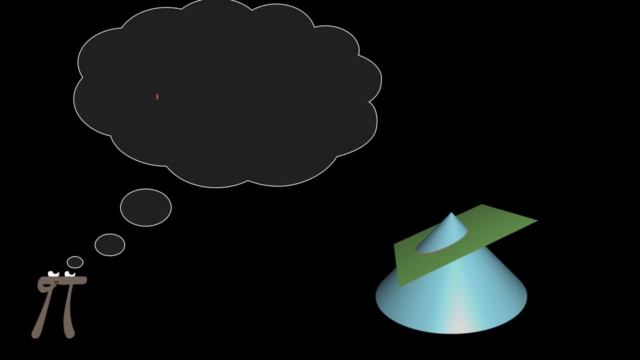 In particular when I was younger. I remember feeling really surprised that slicing a cone would produce such a symmetric shape. You might think that the part of the intersection farther down would kind of bulge out and produce a more lopsided egg shape. 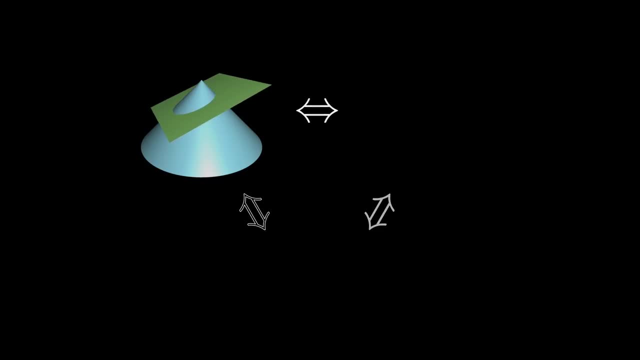 But nope, The intersection curve is an ellipse, the same, evidently symmetric curve you'd get by just stretching a circle or tracing around two thumbtacks. But why should the family of curves produced by these three totally different methods be precisely the same shapes? 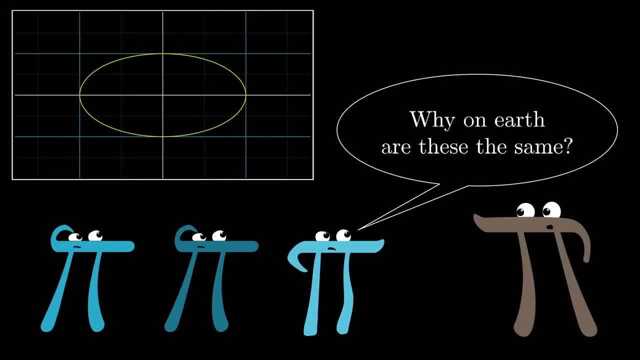 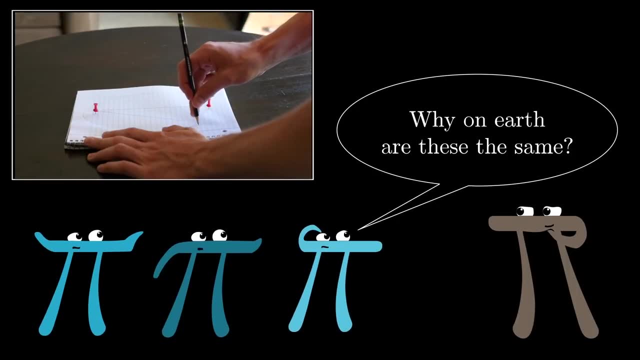 should these three definitions have anything to do with each other? I mean sure it kind of makes sense that each should produce some vaguely oval-looking stretched out loop, but why should the family of curves produced by these three totally different methods be precisely the same shapes? 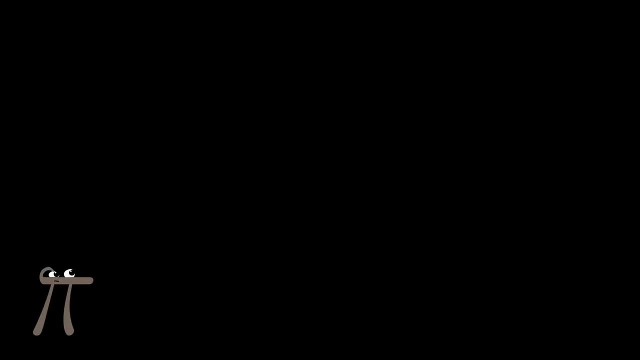 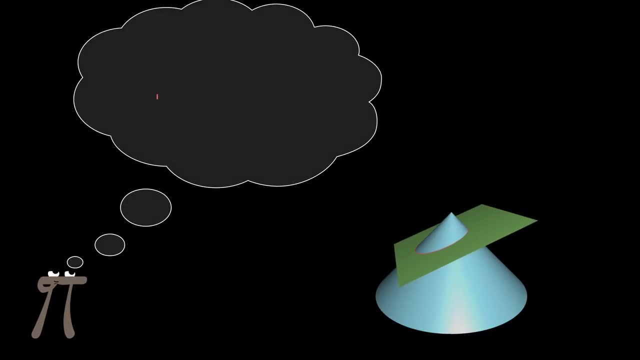 In particular when I was younger. I remember feeling really surprised that slicing a cone would produce such a symmetric shape. You might think that the part of the intersection farther down would kind of bulge out and produce a more lopsided egg shape. 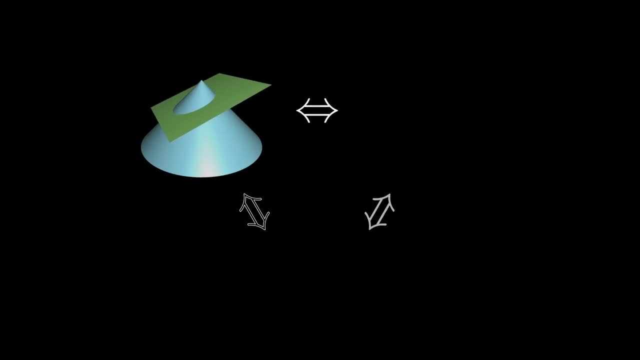 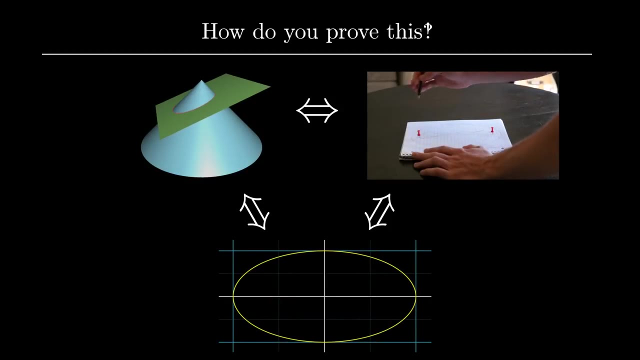 But nope, The intersection curve is an ellipse, the same evidently symmetric curve you'd get by just stretching a circle or tracing around two thumbtacks. But of course math is all about proofs. So how do you give an airtight demonstration that these three families of curves are actually? 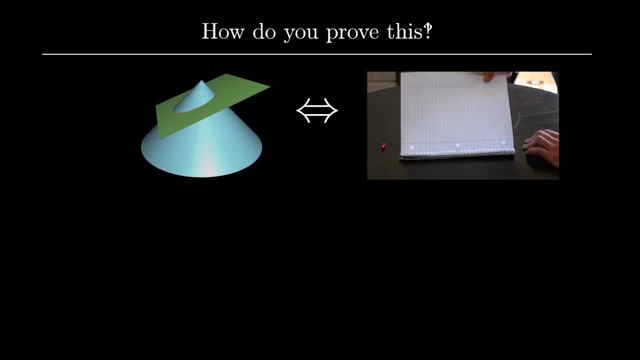 the same. For example, let's focus our attention on just one of these equivalences, namely that slicing a cone will give us a curve that could also be drawn using the thumbtack construction. What you need to show here is that there exist two thumbtack points somewhere inside that. 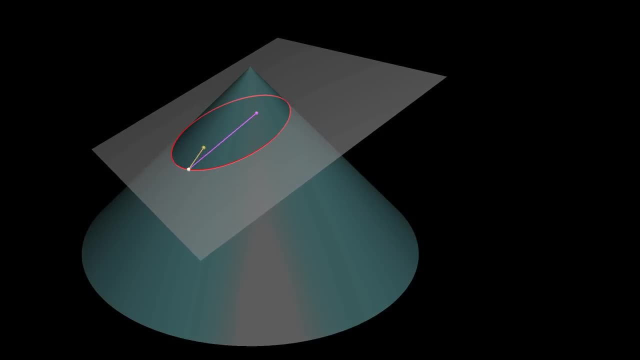 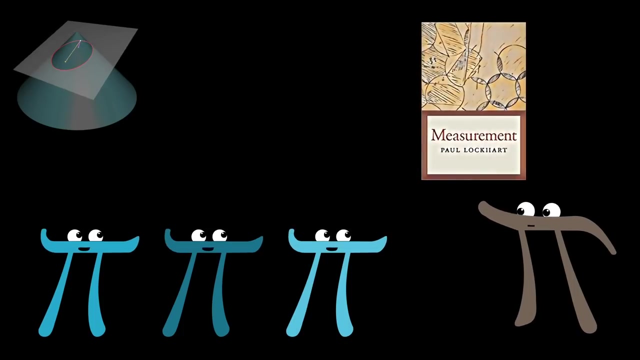 slicing plane such that the sum of the distances from any point of the intersection curve to those two points remains the same. I first saw the trick to showing why this is true in Paul Lockhart's magnificent book Measurement, which I would highly recommend to anyone, young or old, who needs a reminder. 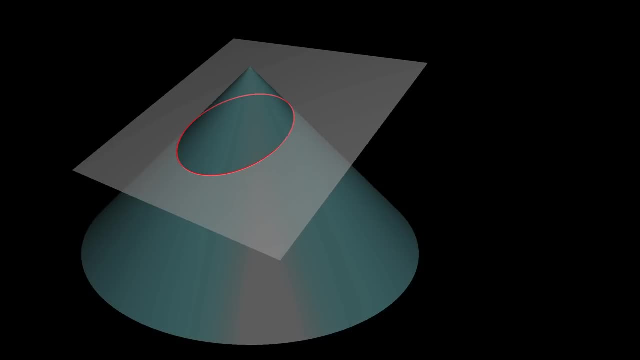 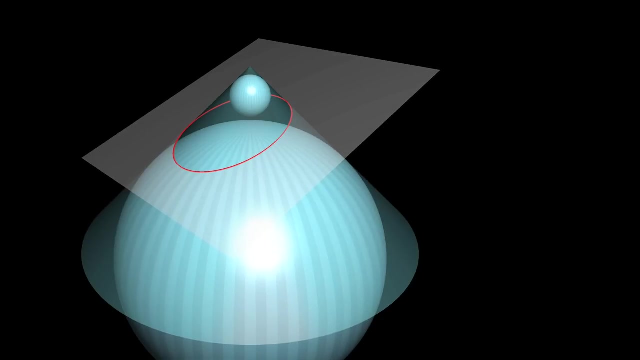 of the fact that math is a form of art. The stroke of genius comes in the very first step, which is to introduce two spheres into this picture, one above the plane and one below it, Each one of them sized just right so as to be tangent to the cone along a circle of points. 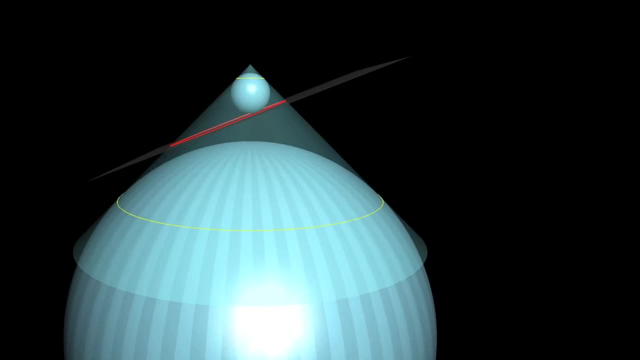 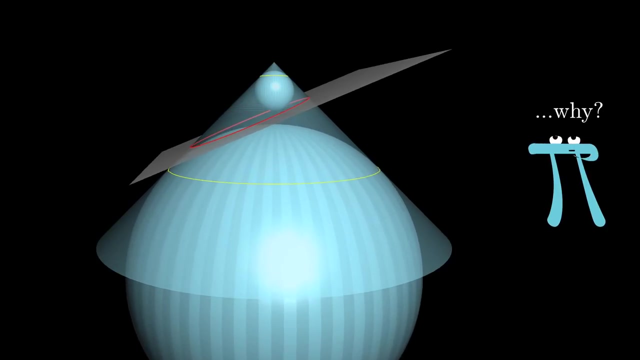 and tangent to the plane along a circle of points. Why you would think to do this, of all things, is a tricky question to answer, and one that we'll turn back to. For right now, let's just say that you have a particularly playful mind that loves engaging. 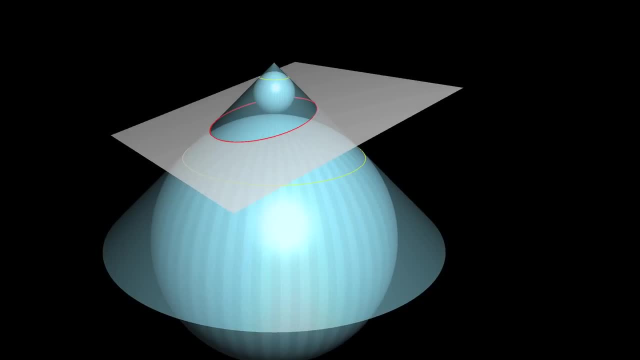 with how different geometric objects all fit together. But once these spheres are sitting here, I actually bet that you could prove the target result yourself Here. I'll help you step through it, but at any point, if you feel inspired, please do. 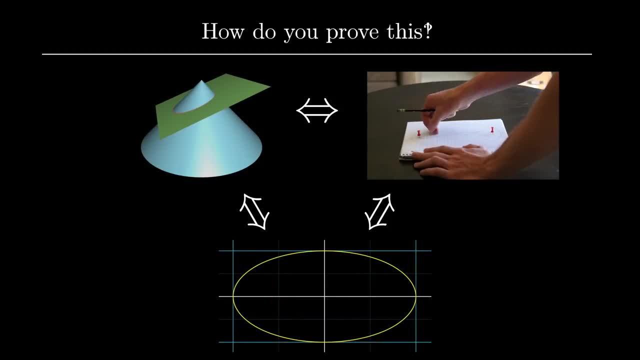 I mean sure it kind of makes sense that these three totally different methods be precisely the same shapes. But why should the family of curves produced by these three totally different methods be precisely the same shapes? But of course math is all about proofs. 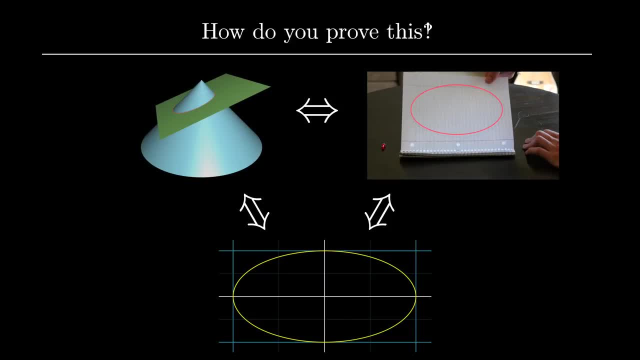 So how do you give an airtight demonstration that these three families of curves are actually the same, For example? let's focus our attention on just one of these equivalences, namely that slicing a cone will give us a curve that could also be drawn using the thumbtack construction. 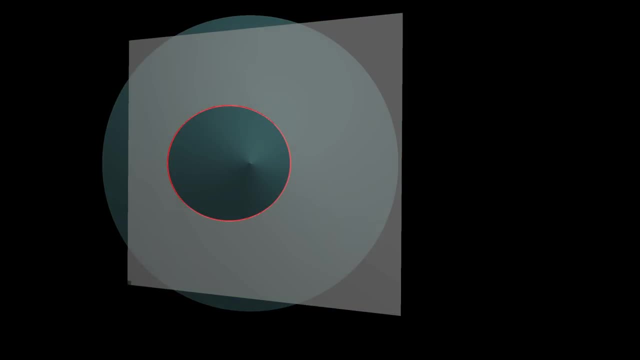 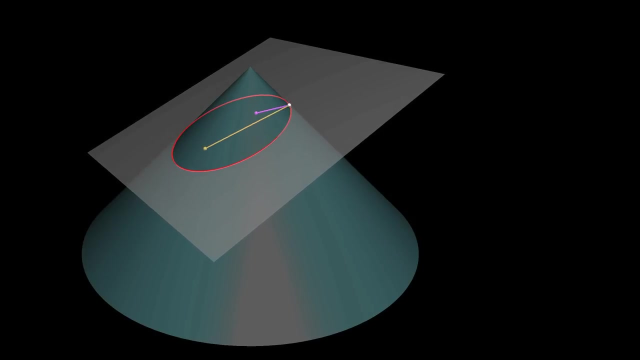 What you need to show here is that there exist two thumbtack points somewhere inside that slicing plane, such that the sum of the distances from any point of the intersection to the point of the intersection curve to those two points remains constant, no matter where. 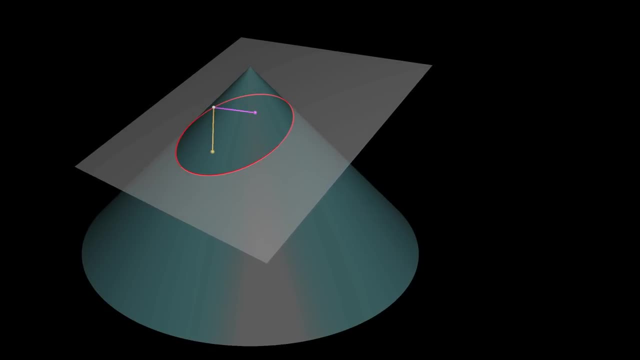 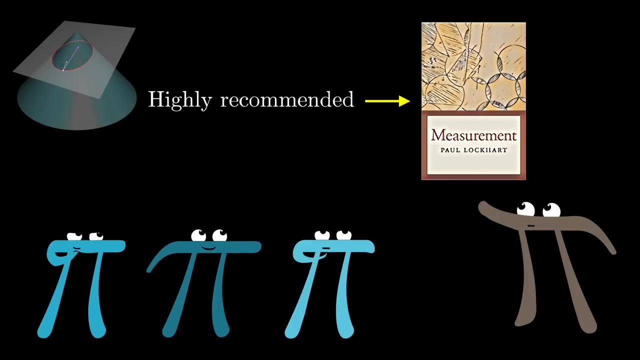 you are on that intersection curve. I first saw the trick to showing why this is true in Paul Lockhart's magnificent book Measurement, which I would highly recommend to anyone, young or old, who needs a reminder of the fact that math is a form of art. 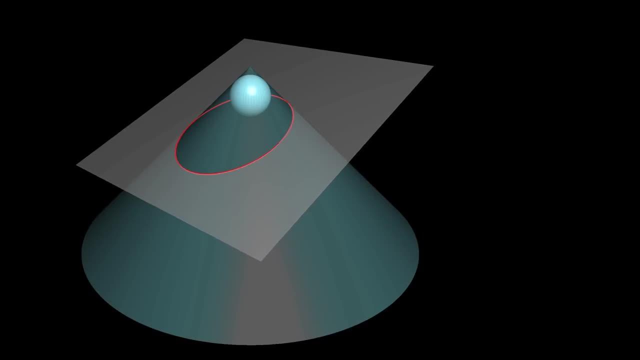 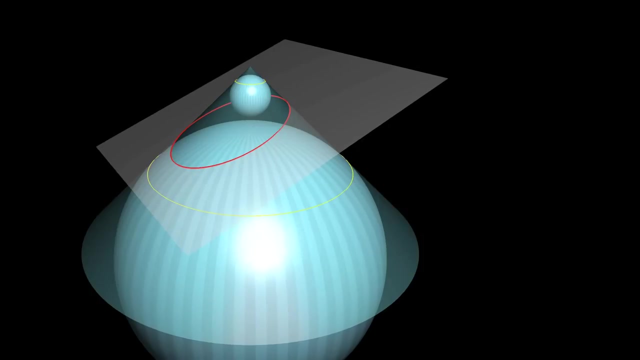 The stroke of genius comes in the very first step, which is to introduce two spheres into this picture, one above the plane and one below it, each one of them sized just right: those to be tangent to the cone along a circle of points and tangent to the plane at just. 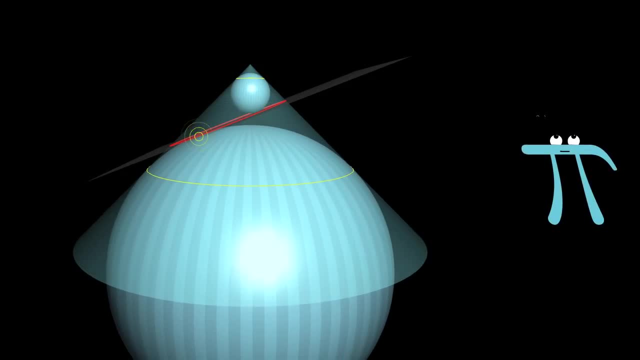 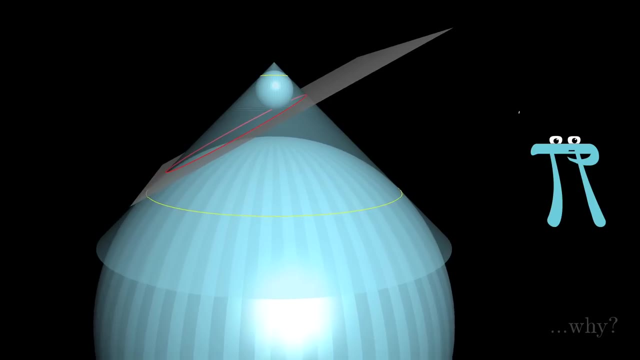 a single point. Why you would think to do this of all things is a tricky question to answer, and one that we'll turn back to. For right now, let's just say that you have a particularly playful mind that loves engaging with how different geometric objects all fit together. 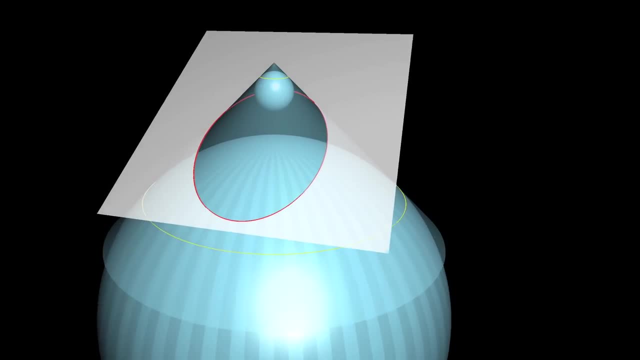 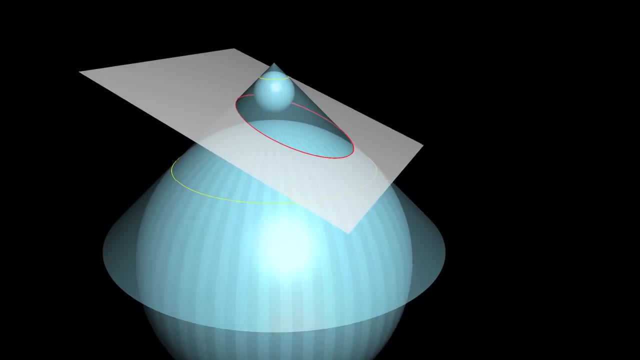 But once these spheres are sitting here, I actually bet that you could prove the target result yourself Here. I'll help you step through it, But at any point, if you feel inspired, please do pause and just try to carry on without me. 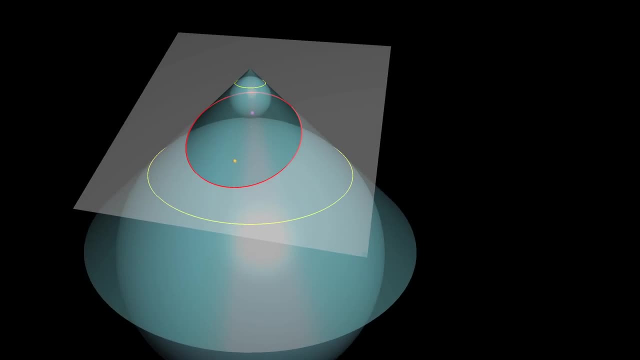 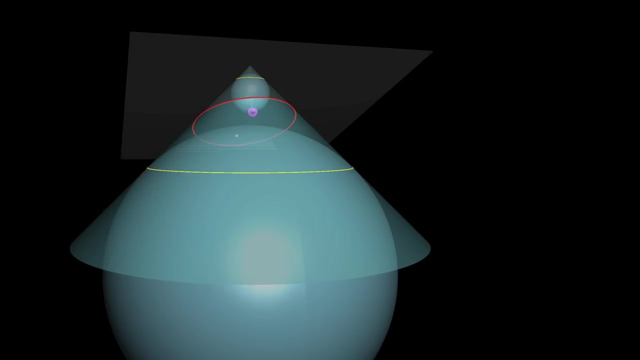 First off, these spheres have introduced two special points inside the curve, the points where they're tangent to the plane. So a reasonable guess might be that these two tangency points are the focus points. That means that you're going to want to draw lines from these foci to some point along. 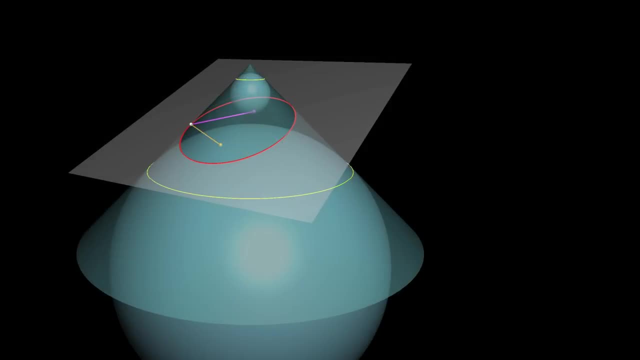 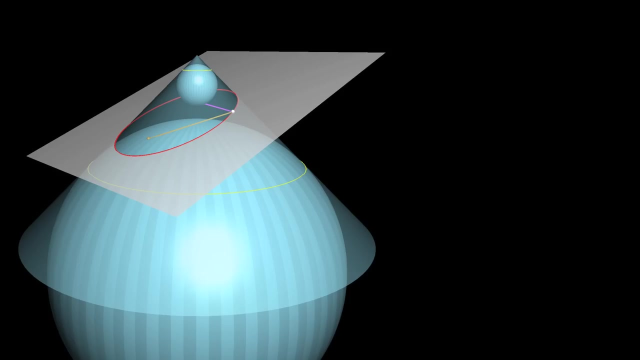 the ellipse and ultimately, the goal is to understand what the sum of the distances of those two lines is, Or, at the very least, to understand why that sum doesn't depend on where you are along the ellipse. Keep in mind: what makes these lines special is that each one does not simply touch one. 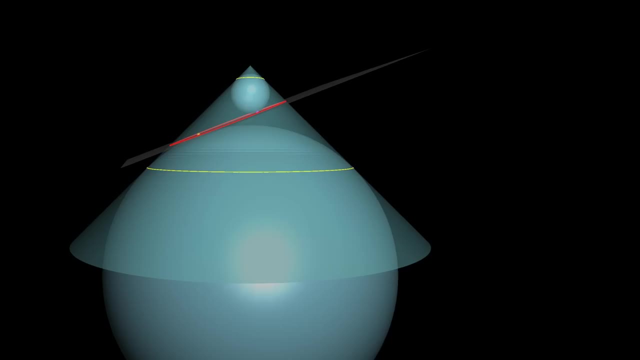 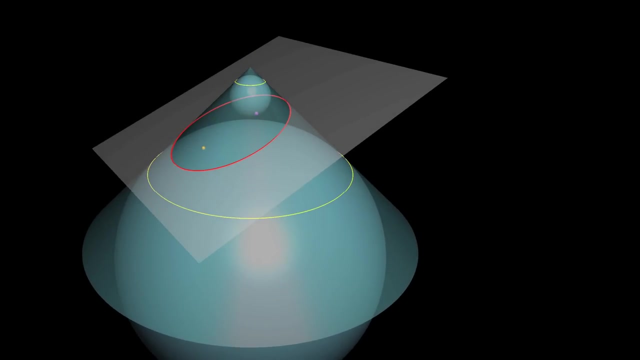 pause and just try to carry on. First off, these spheres have introduced two special points inside the curve, the points where they're tangent to the plane. So a reasonable guess might be that these two tangency points are the focus points. That means that you're going to want to draw lines from these foci to some point along. 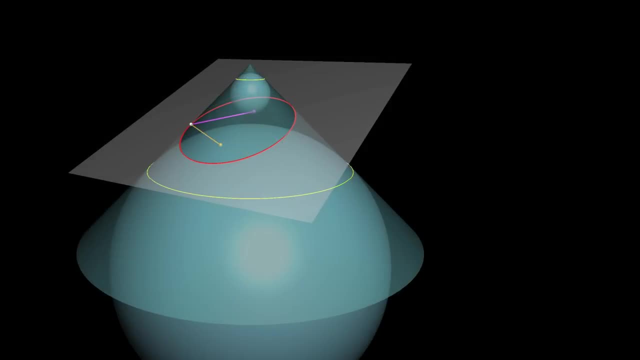 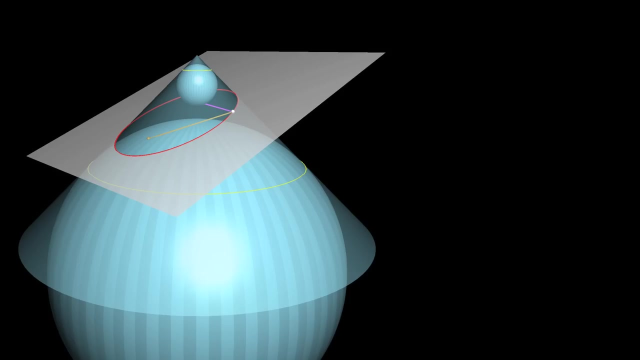 the ellipse and ultimately, the goal is to understand what the sum of the distances of those two lines is, Or, at the very least, to understand why that sum doesn't depend on the distance between these two lines. Keep in mind: what makes these lines special is that each one does not simply touch one. 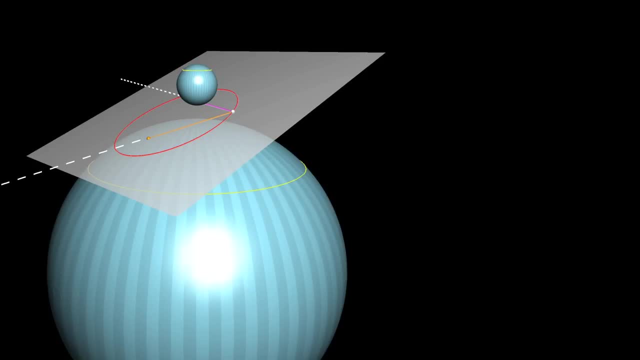 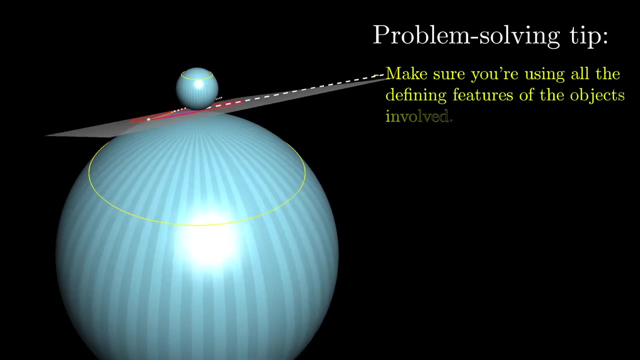 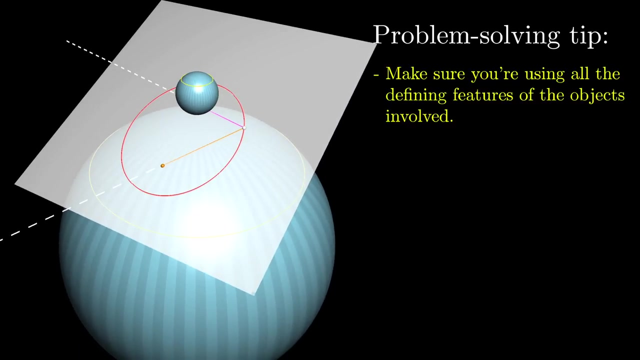 of the spheres. it's actually tangent to that sphere at the point where it touches, And in general for any math problem you want to use the defining features of all the objects involved. Another example here is what even defines the spheres: It's not just the fact that they're tangent to the plane, but that they're also tangent. 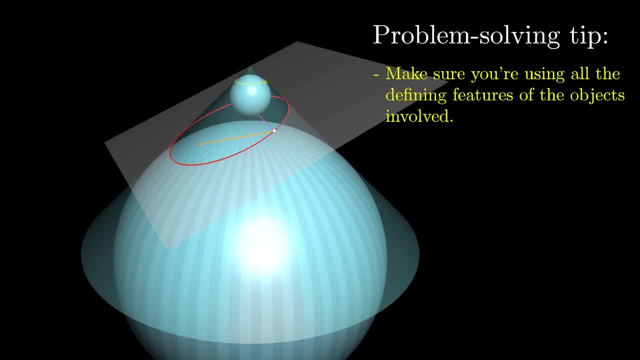 to the cone. It's the circle of tangency points. So you're going to need to use those two circles of tangency points in some way, But how exactly? One thing you might do is just draw a line straight from the top circle down to the bottom. 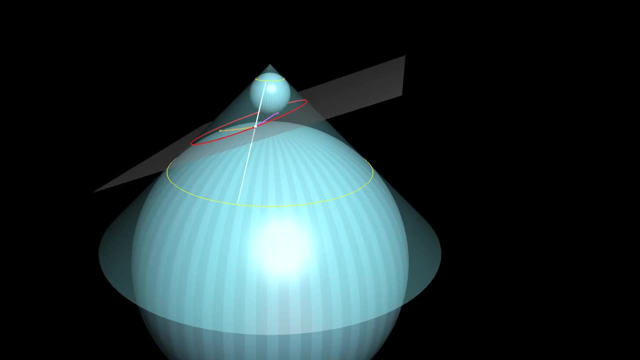 one along the cone, And there's something about doing this that feels vaguely reminiscent of the constant sum thumbtack property and hence promising. It passes through the ellipse, and so, by snipping that line at the point where it crosses the ellipse, you can think of it as the sum of two line segments, each one hitting the same. 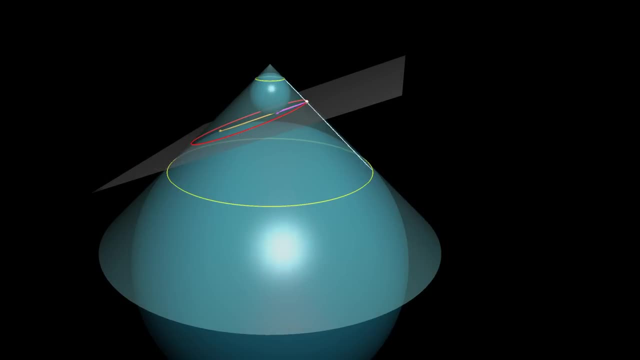 point on the ellipse- And you can do this through various different points of the ellipse depending on where you are around the cone- always getting two line segments with a constant sum, namely whatever the straight line distance from the top circle to the bottom circle is. 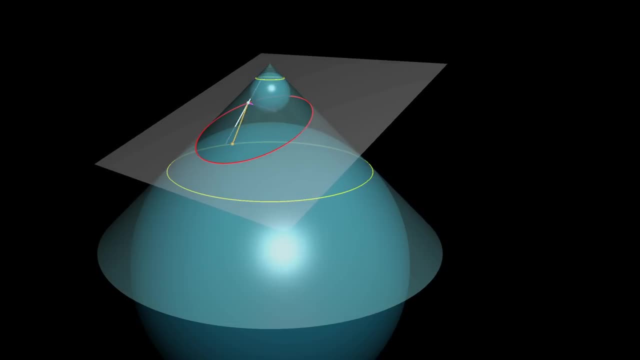 So you see what I mean about it being vaguely analogous to the thumbtack property, in that every point of the ellipse gives us two distances whose sum is a constant. Granted, these lengths are not to the focal points, but maybe that leads you to making 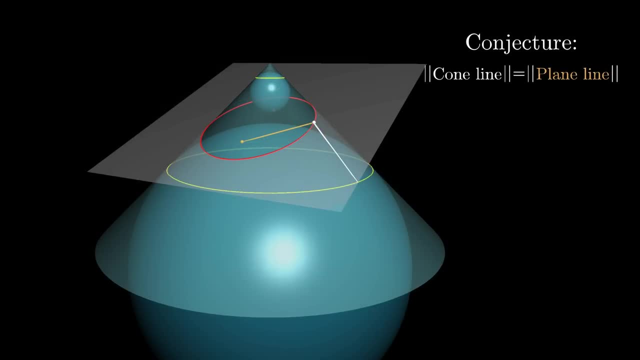 the following conjecture: The distance from a given point on this ellipse, this intersection curve straight down to the big circle, is, you conjecture, equal to the distance to the point where that big sphere is tangent to the plane, our first proposed focus point. 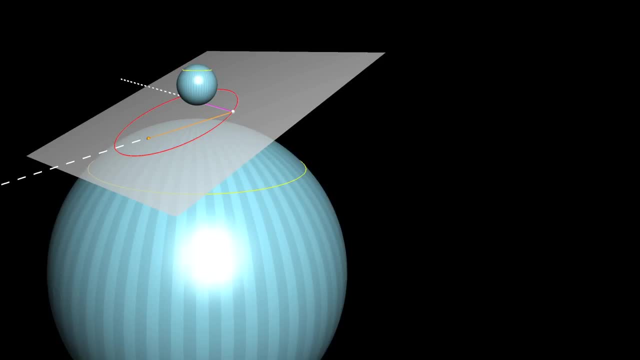 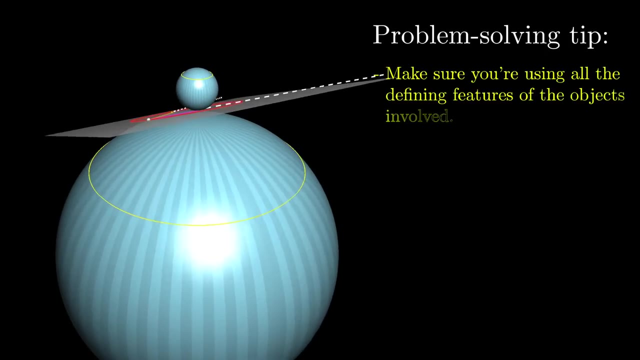 of the spheres. it's actually tangent to that sphere at the point where it touches, And in general for any math problem you want to use the defining features of all of the objects involved. Another example here is what even defines the spheres. It's not just the fact that they're tangent. 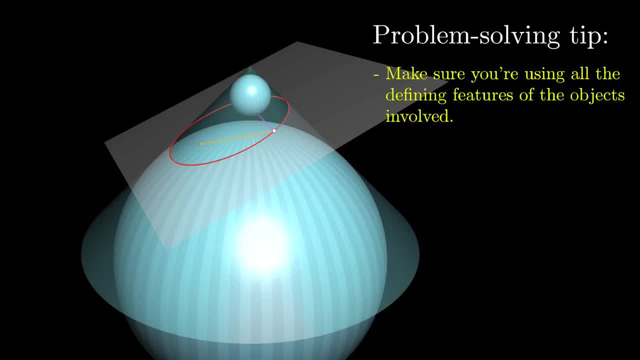 It's that they're tangent to the plane, But that they're also tangent to the cone, each one at some circle of tangency points. So you're going to need to use those two circles of tangency points in some way, But how exactly? 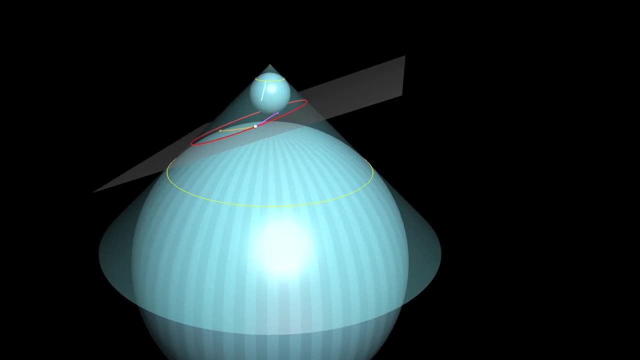 Well, one thing you might do is just draw a line straight from the top circle down to the bottom one along the cone, And there's something about doing this that feels vaguely reminiscent of the constant sum thumbtack, property and hence promising. You see, it passes through the cone. 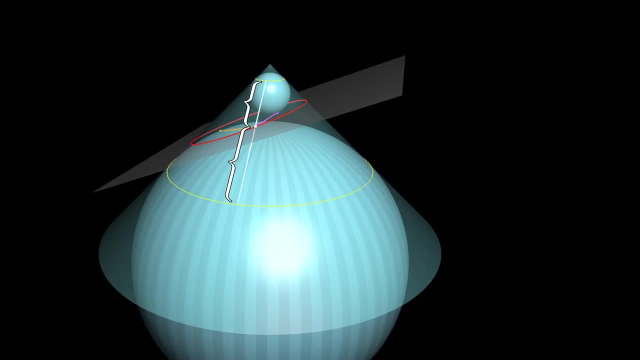 It passes through the cone, It passes through the ellipse, And so, by snipping that line at the point where it crosses the ellipse, you can think of it as the sum of two line segments, each one hitting the same point on the ellipse. 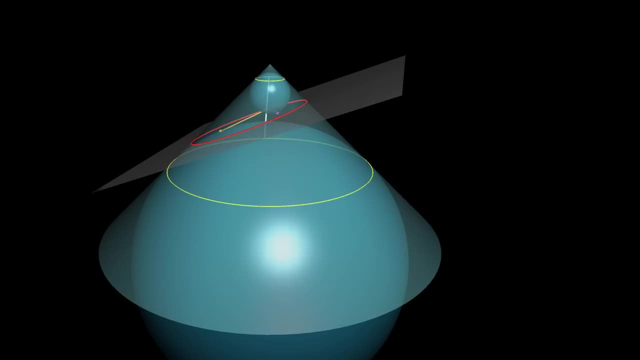 And you can do this through various different points of the ellipse, depending on where you are around the cone, always getting two line segments with a constant sum, namely whatever the straight line distance from the top circle to the bottom circle is. So you see what I mean about it being vaguely analogous to the thumbtack property in that 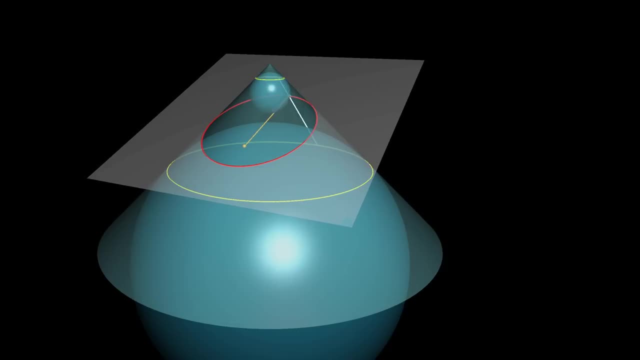 case, you just need to don the turn backtack and you have a full circle that ends on the bottom circle. Further, you say that the point of the cone on the top circle in the ellipse is the point with the formula I just described. 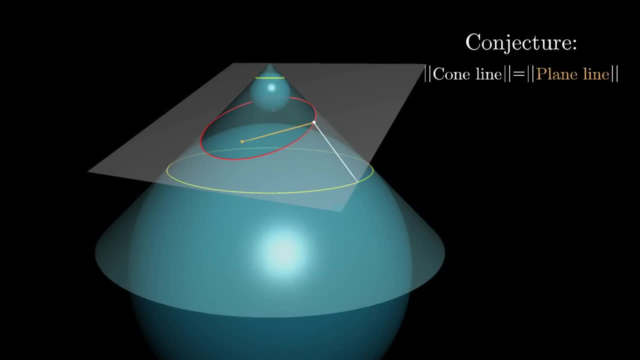 And this is the entrevist who said that when the cone is broken in half- and is not only the point of the cone but the whole circle that's broken down- is the point on the top circle. He gives us two distances from each point on the ellipse, whose sum is a constant. 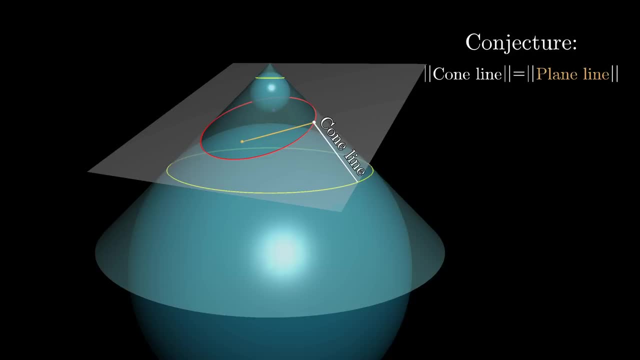 Granted, these lengths are not to the focal point, but maybe that leads us to making the following conjecture: The distance from a given point on this ellipse straight down to the big circle is equal to the distance to the point where that big sphere is tangent to the plane. 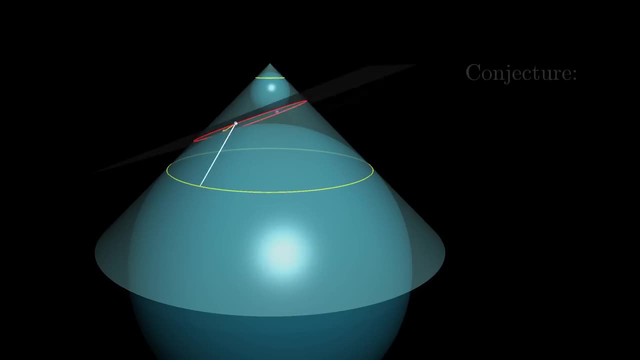 Likewise, perhaps the distance from that point on the ellipse is the distance from the cone. Likewise, perhaps the distance from that point on the ellipse to the small circle is equal to the distance from that point to the second proposed focus point, where the small sphere. 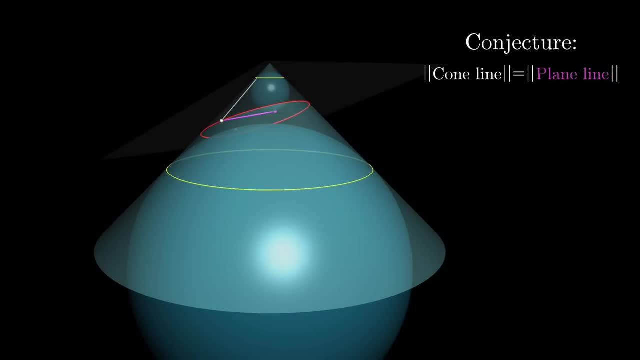 Likewise, perhaps the distance from that point on the ellipse to the small circle is equal to the distance from that point to the small circle, So you can think of this as the sum of two line segments, and so on. So is that true? 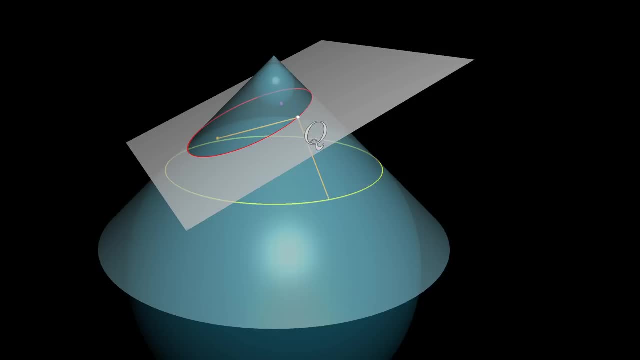 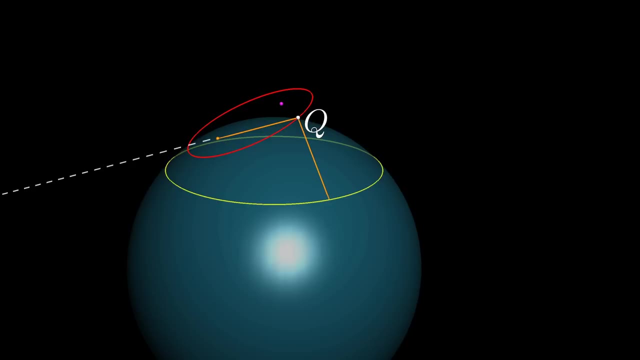 Well, yes, Here let's give a name to that point. on the ellipse q, The key is that the line from q to the first proposed focus is tangent to the big sphere and the line from q straight down along the cone is also tangent to the big sphere. 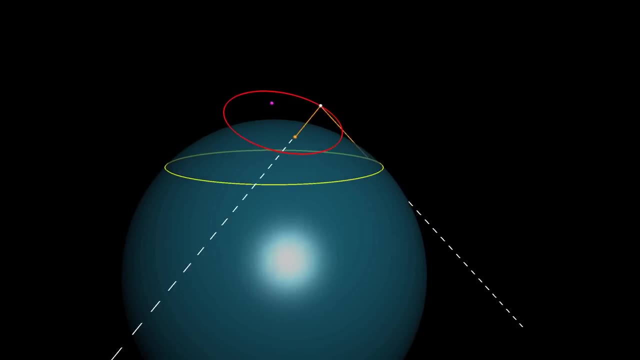 Here let's look at a different picture for some clarity. If you have multiple lines drawn from a common point to a sphere, then the line from q to the first proposed focus is tangent to the big sphere. So here let's look at a different picture for some clarity. 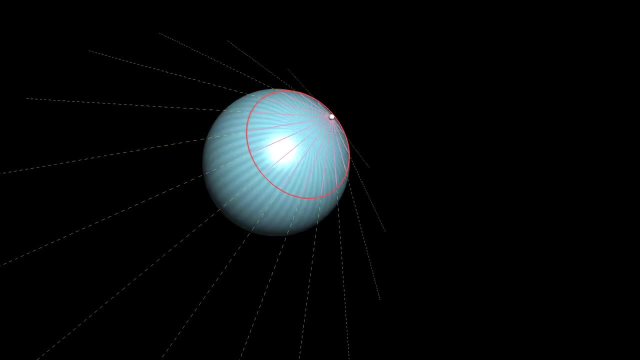 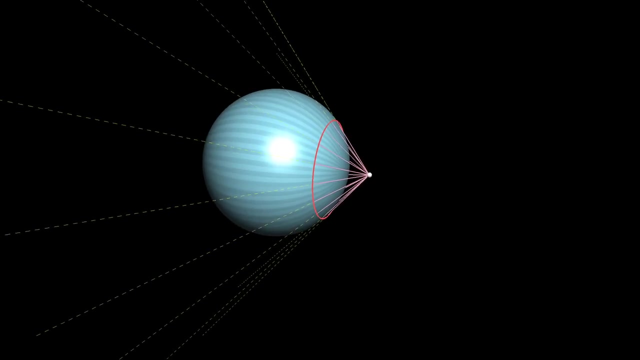 All of which are tangent to that sphere. you can probably see just from the symmetry of the setup that all of those lines have to have the same length, And in fact I encourage you to try proving this yourself or to otherwise. pause and ponder. 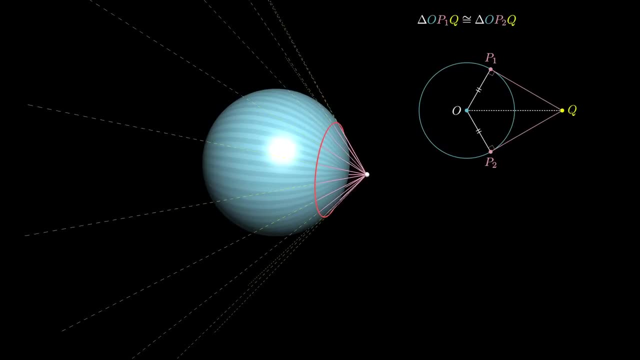 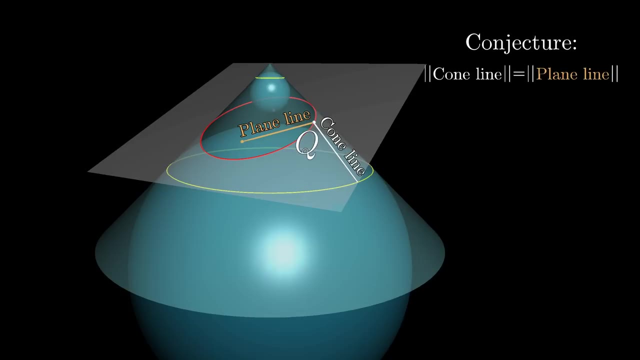 on the proof that I've left on this screen, But looking back at our cone slicing setup, your conjecture would be correct. the two lines extending from point Q to the ellipse tangent to the big sphere each have the same length. Similarly, the line from q to the first proposed focus is tangent to the sphere. 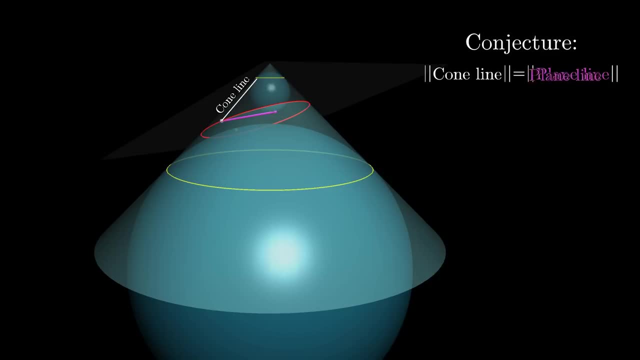 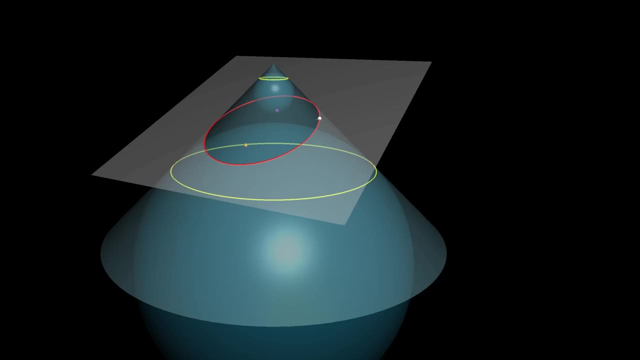 So for all, clear here is that these two points, tangent, from Q to the first proposed focus, to the second proposed focus point, is tangent to the little sphere, as is the line from Q straight up along the cone, so those two also have the same length And so the sum of the 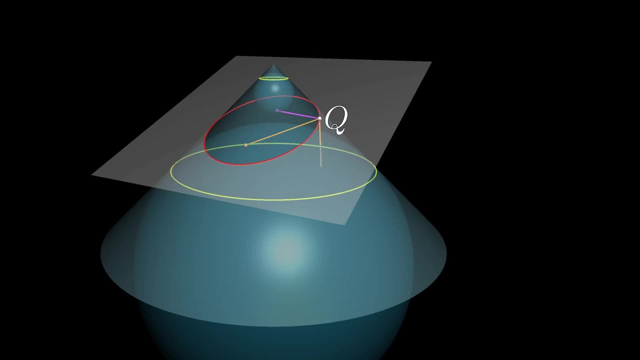 distances from Q to the two proposed focus points is the same as the straight line distance from the little circle down to the big circle along the cone passing through Q, And clearly that does not depend on which point of the ellipse you chose for Q. Bada-boom-bada-bang slicing the cone. 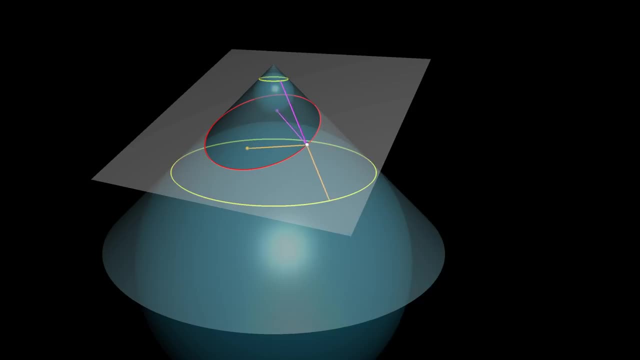 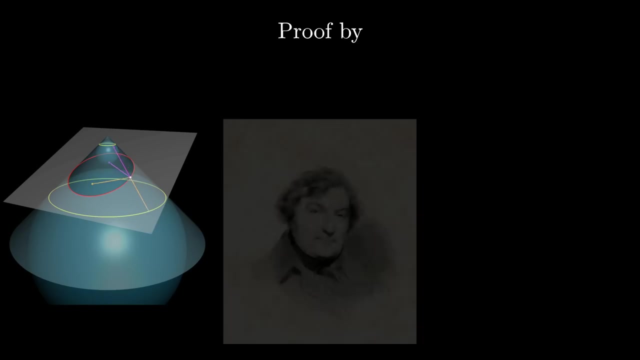 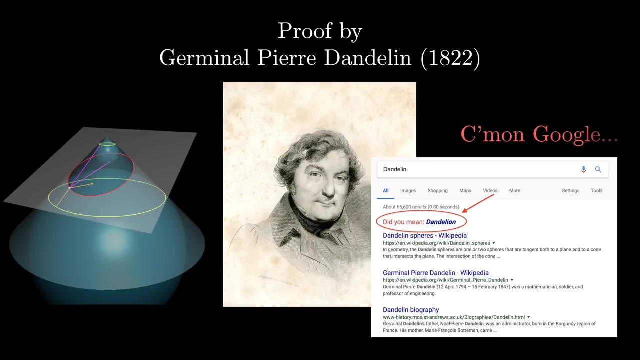 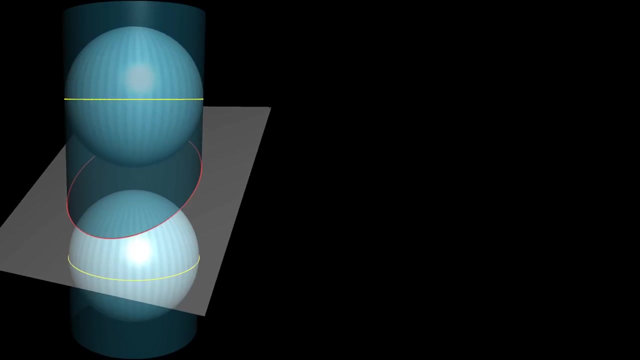 is the same as the thumbtack construction, since the resulting curve has the constant focal sum property. Now, this proof was first found by Dandelion, a guy named Dandelion, in 1822.. So these two spheres are sometimes called Dandelion spheres. You can also use the same trick to show: 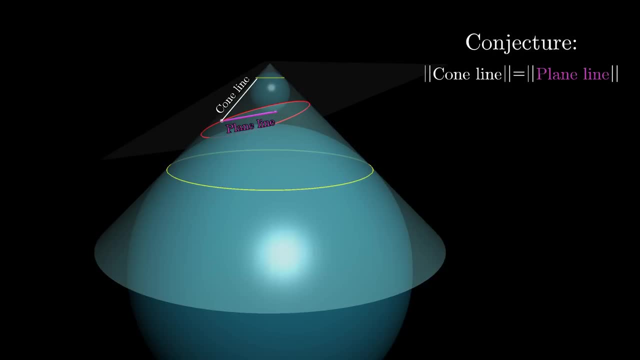 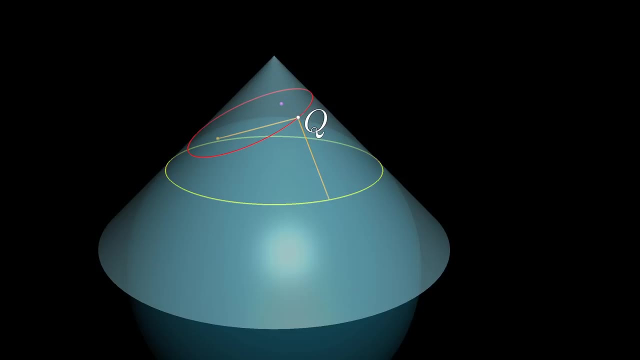 touches the plane. So is that true? Well, yes, Here let's give a name to that point. on the ellipse Q, The key is that the line from Q to the first proposed focus is tangent to the big sphere and the line from Q straight. 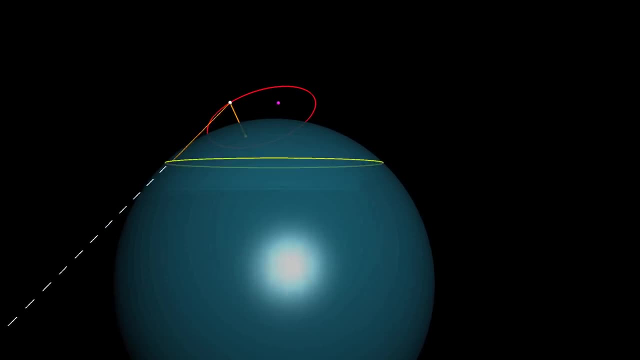 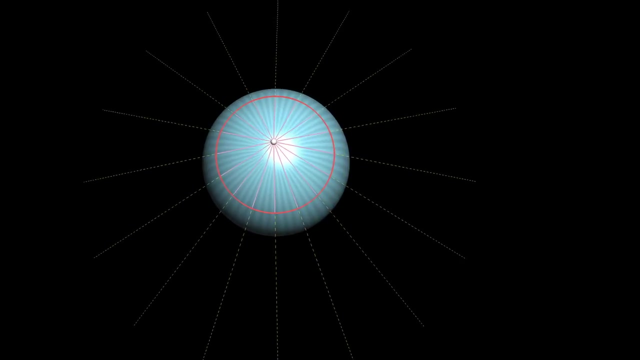 down along the cone is also tangent to the big sphere. Here let's look at a different picture for some clarity. If you have multiple lines drawn from a common point to a sphere, all of which are tangent to that sphere, you can probably see just from the symmetry of the setup that all of 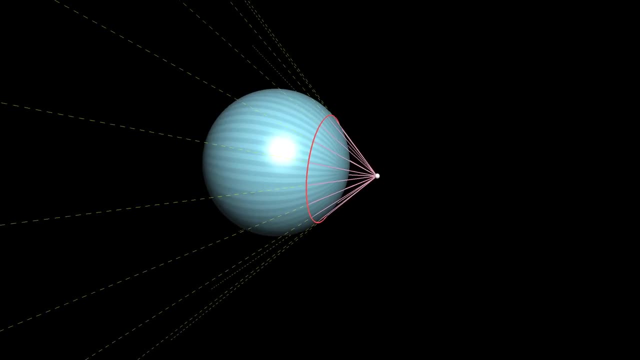 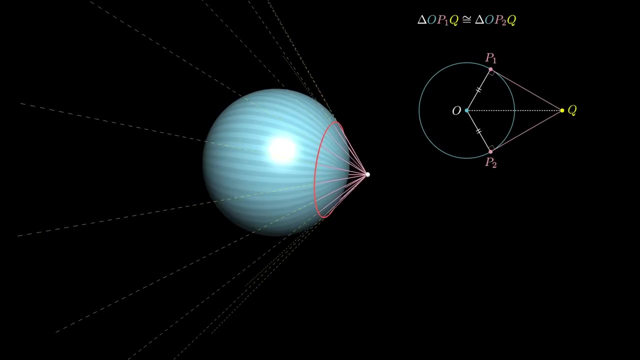 these lines have to have the same length. In fact, I encourage you to try proving this yourself, or to otherwise. pause and ponder on the proof I've left on the screen. But looking back at our cone slicing setup, Your conjecture would be correct. 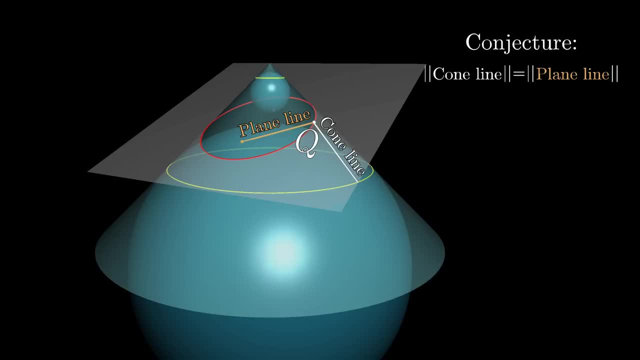 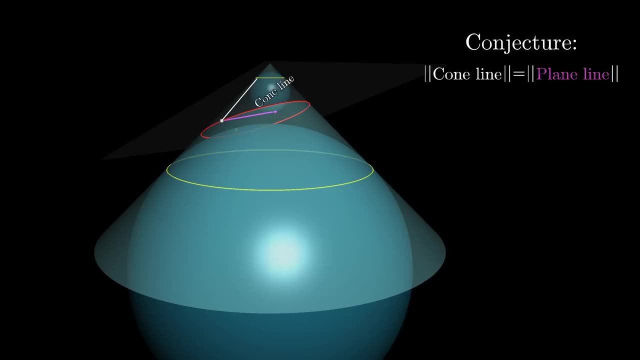 The two lines extending from the point Q on the ellipse tangent to the big sphere have the same length. Similarly, the line from Q to the second proposed focus point is tangent to the little sphere, as is the line from Q straight up along the cone. so those two also have the same length. 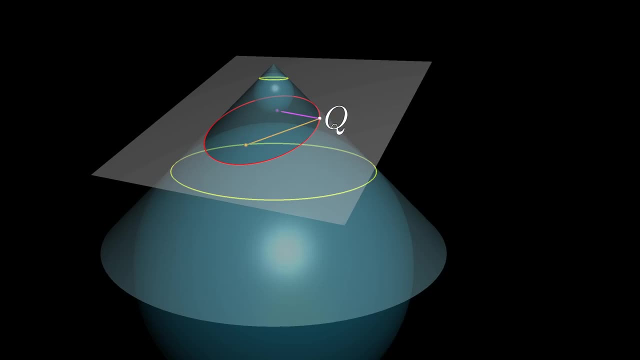 And so the sum of the distances from Q to the two proposed focus points is the same as the straight line distance from the little circle down to the big circle, And clearly that does not depend on which point of the ellipse you chose for Q. 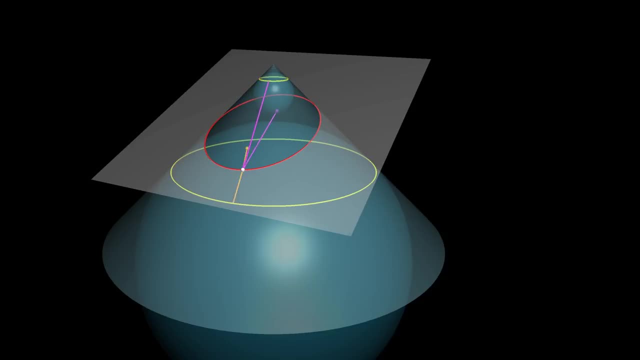 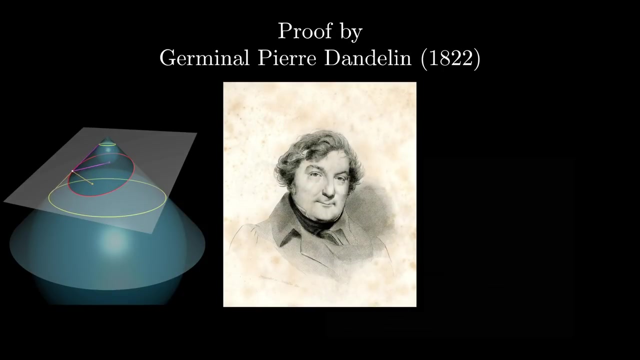 Bada, boom, bada bang. slicing the cone is the same as the thumbtack construction, since the resulting curve has the constant focal sum property. This proof was first found by Dandelion, a guy named Dandelion, in 1822, so these two. 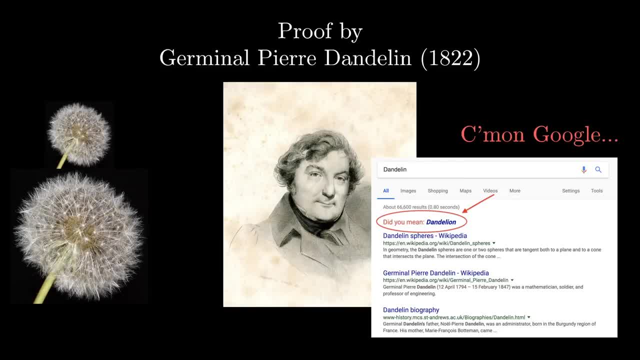 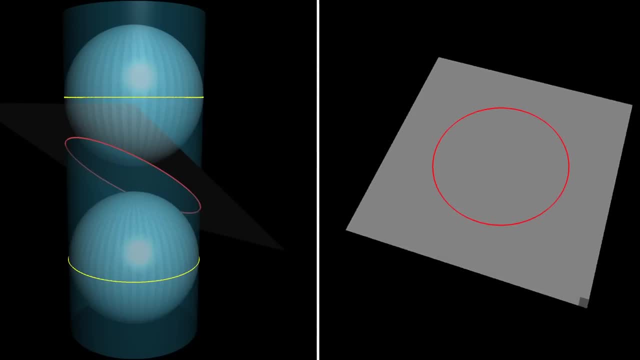 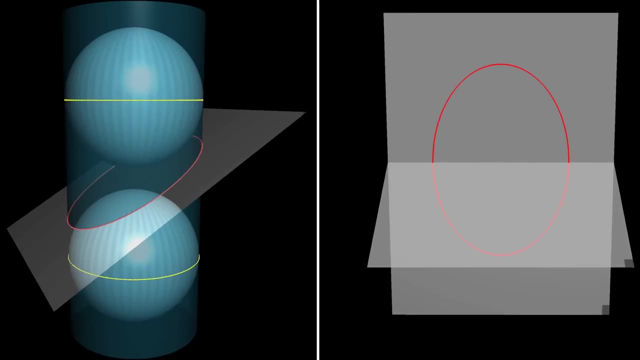 spheres are sometimes called dandelions. You can also use the same trick to show why slicing a cylinder at an angle will give you an ellipse. and if you're comfortable with the claim that projecting a shape from one plane onto another tilted plane has the effect of simply stretching out that shape, this 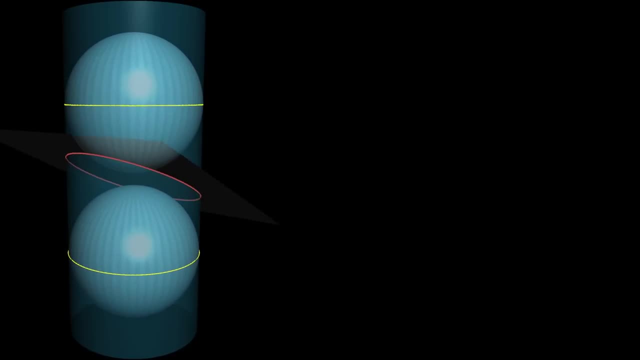 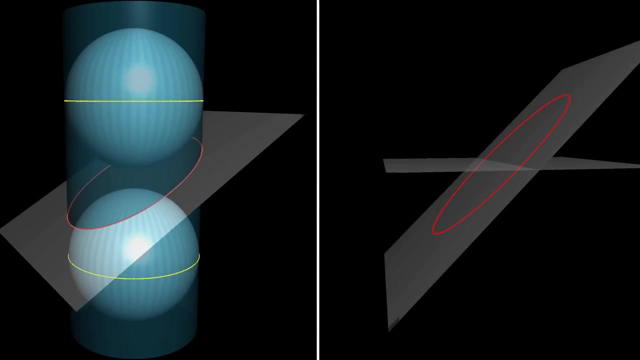 why slicing a cylinder at an angle will give you an ellipse. And if you're comfortable with the claim, you can also use the same trick to show why slicing a cylinder at an angle will give you an ellipse. This also shows why the definition of an ellipse as a stretched circle is the same. 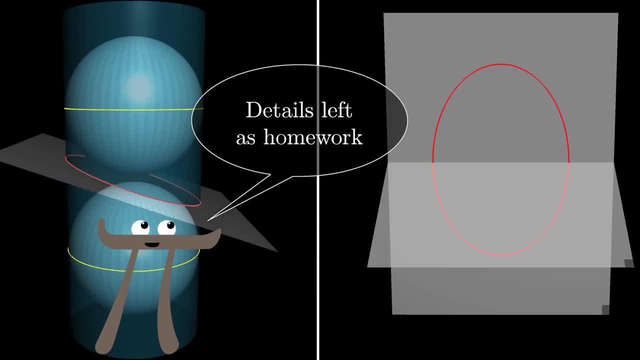 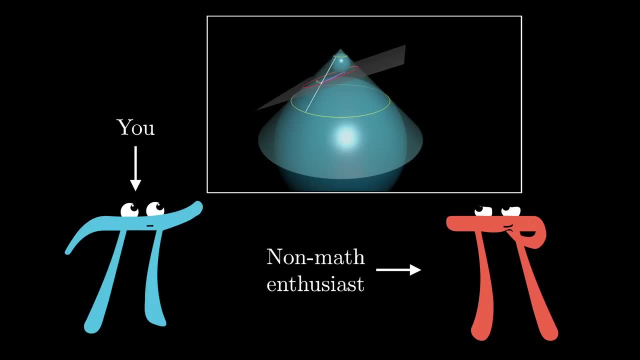 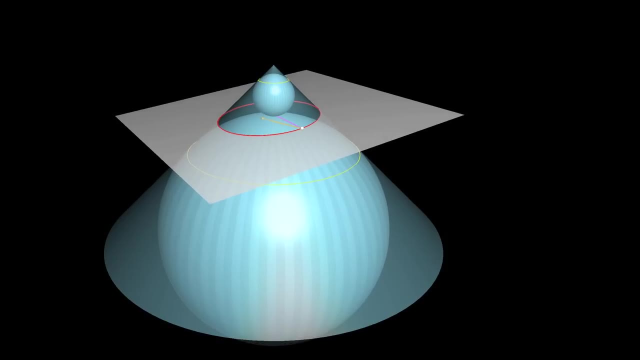 as the other two, More homework. So why do I think that this proof is such a good representative for math itself That if you had to show just one thing to explain to a non-math enthusiast why you love the subject, why this would be a good candidate? The obvious reason is that it's 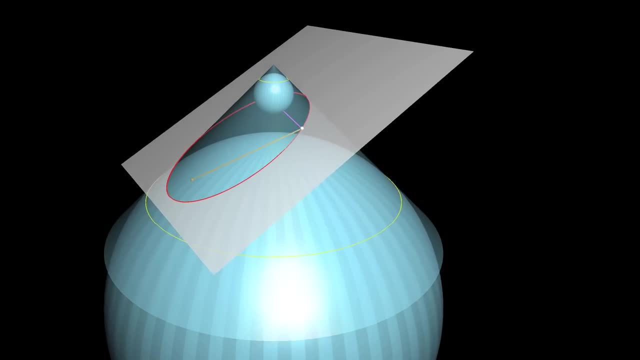 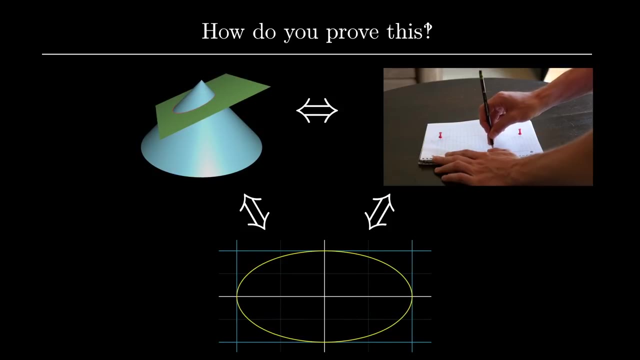 substantive and beautiful without requiring too much background. But more than that, it reflects a common feature of math: that sometimes there is no single, most fundamental way of defining something. That what matters more is showing equivalences And, even more than that, the proof. 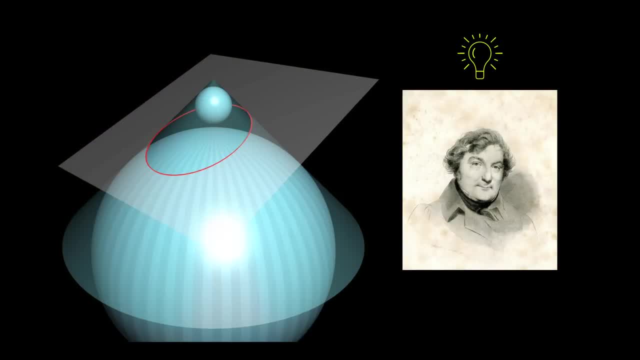 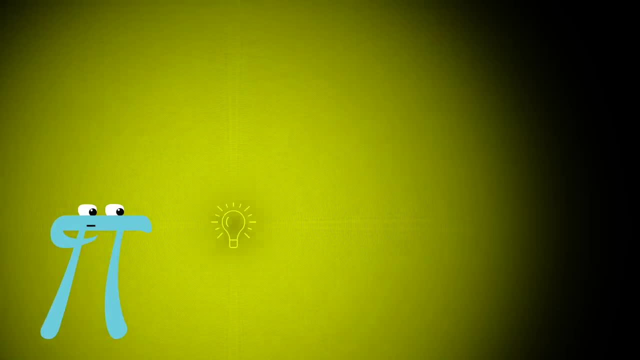 itself involves one key moment of creative construction: adding the two spheres, while most of it leaves room for a nice, systematic and principled approach, And this kind of creative construction is, I think, one of the most thought-provoking aspects of math. 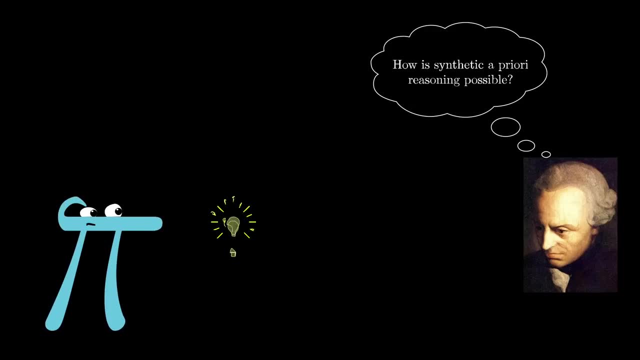 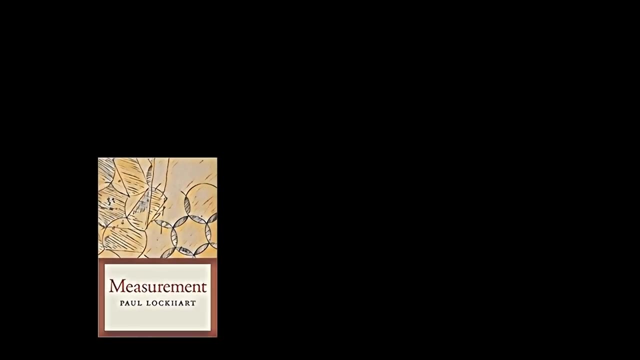 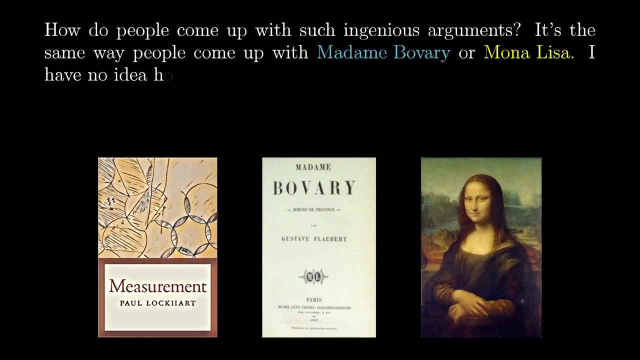 And you might understandably ask where such an idea comes from. In fact, talking about this particular proof, here's what Paul Lockhart says: in Measurement, How do people come up with such ingenious arguments? It's the same as the way people come up with Madame Bovary or Mona Lisa. I have no idea how it happens. I only know that when 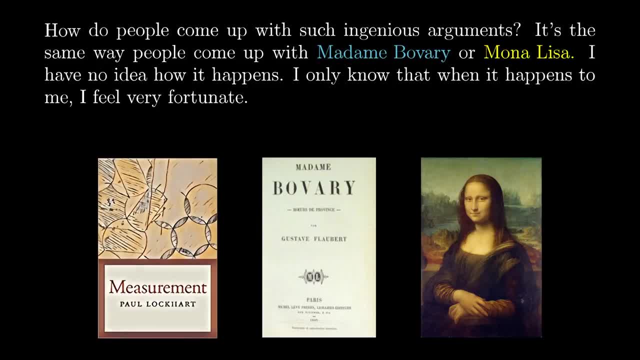 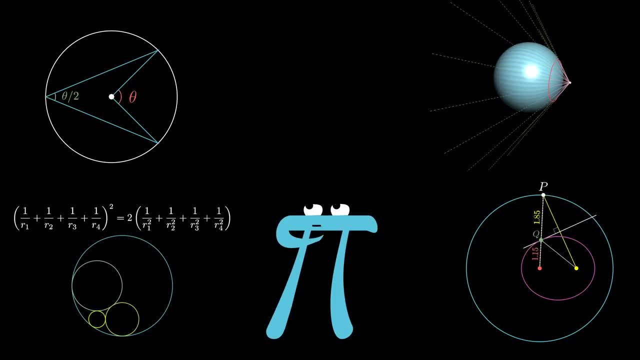 it happens to me. I feel very fortunate. I agree, but I do think we can say at least a little something more about this. While it is ingenious, we can perhaps decompose something, And this is how someone who has immersed themselves in a number of other geometry problems might. 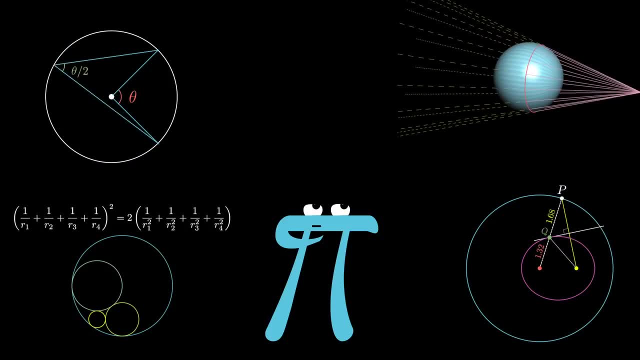 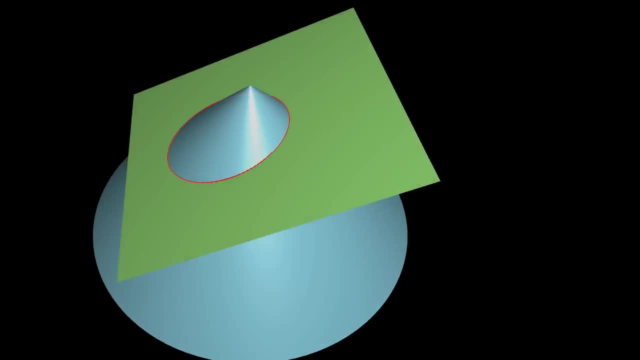 be particularly primed to think of adding these specific spheres. First, a common tactic in geometry is to relate one length to another And in this problem you know from the outset that being able to relate these two lengths to the foci, to some other two lengths especially, 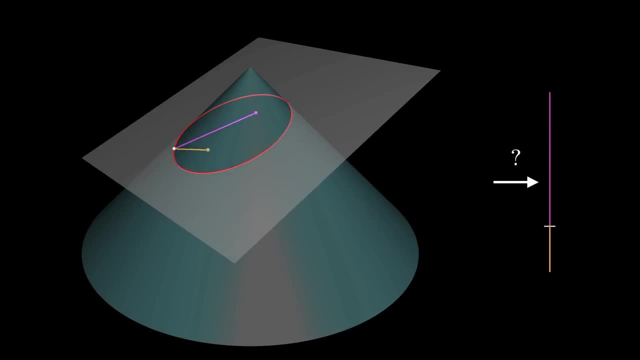 ones. that line up would be a useful thing, Even though at the start you don't even know where the focus points are. But if we were able to do that, we could be more accurate at solving this problem And from this point on we could have been able to gather all of the other spheres in a linear. 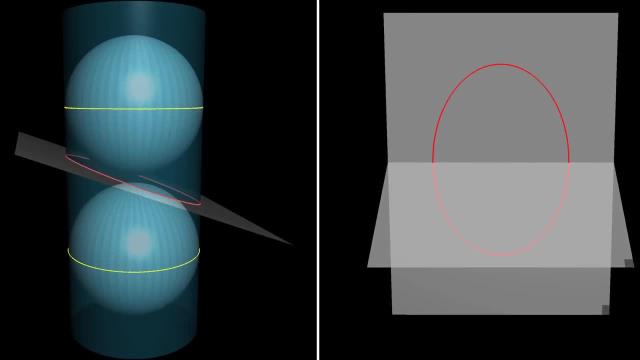 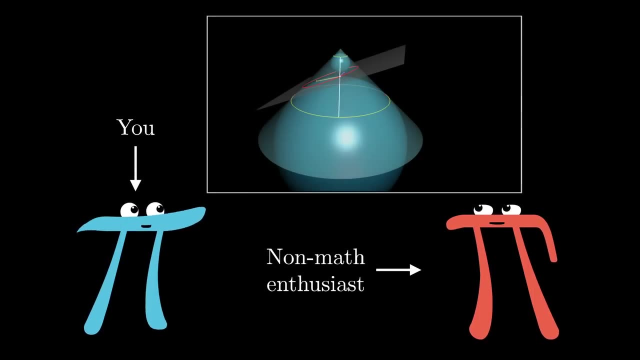 also shows why the definition of an ellipse as a stretched circle is the same as the other two. More homework. So why do I think this proof is such a good representative for math itself that, if you had to show just one thing to explain to a non-math enthusiast why you love the subject? 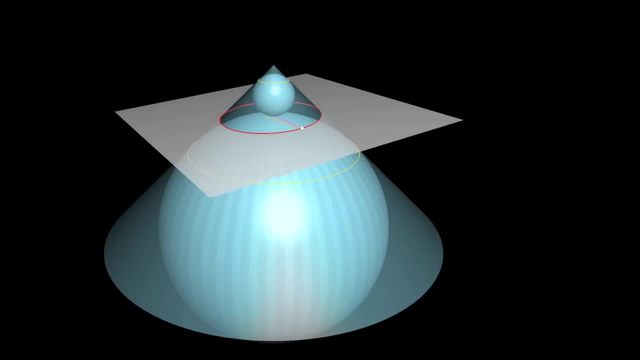 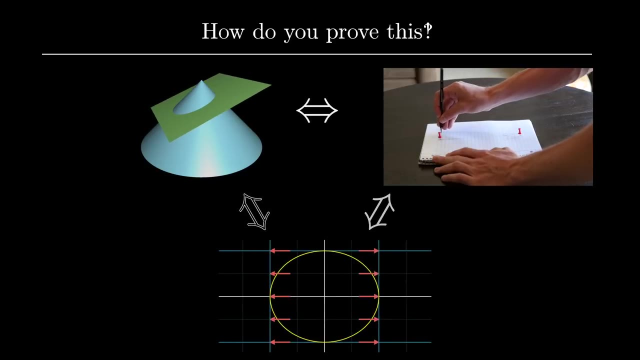 why this would be a good candidate. The obvious reason is that it's substantive and beautiful without requiring too much background. But more than that, it reflects a common feature of math: that sometimes there is no single, most fundamental way of defining something, that what matters more is showing equivalences. 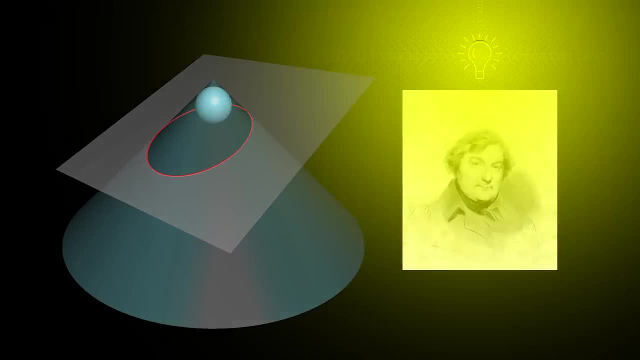 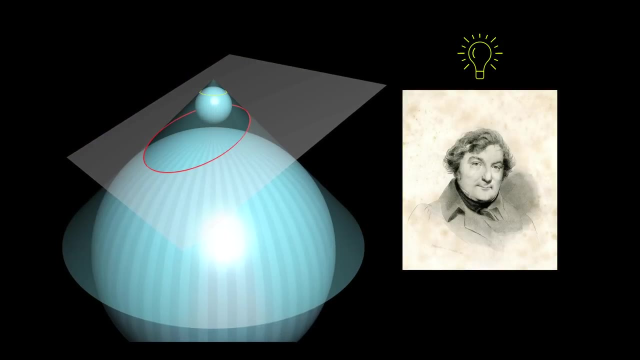 And even more than that. the proof itself involves one key moment of creative construction: adding the two spheres, While most of it leaves room for a nice, systematic and principled approach, And this kind of creative construction is, I think, one of the most thought-provoking. 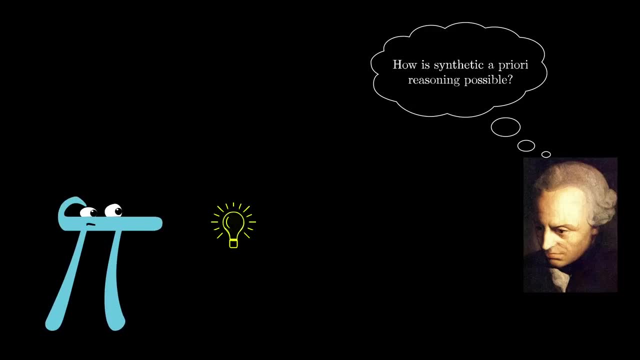 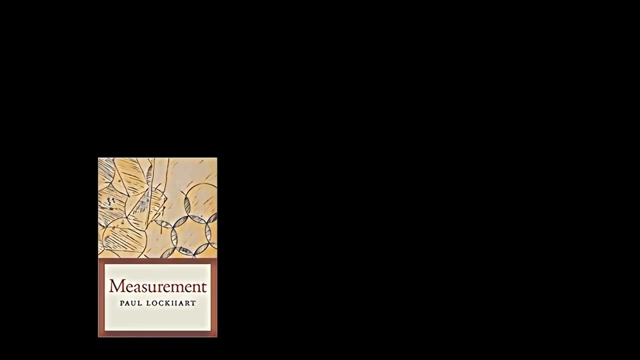 aspects of mathematical discovery, and you might understandably ask where such an idea comes from. In fact, talking about this particular proof, here's what Paul Lockhart says: in Measurement, How do people come up with such ingenious arguments? It's the same as the way people come up with Madame Bovary or Mona Lisa. 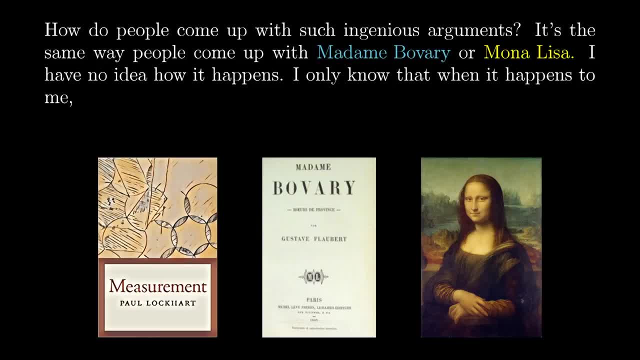 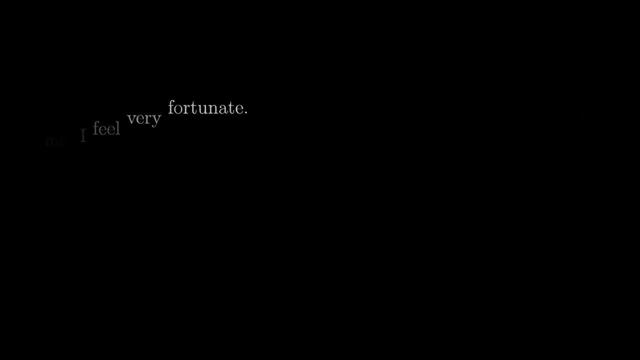 I have no idea how it happens. I only know that when it happens to me, I feel very fortunate. I agree, but I do think we can say at least a little something more about this. While it is ingenious, we can perhaps decompose how someone who has immersed themselves in 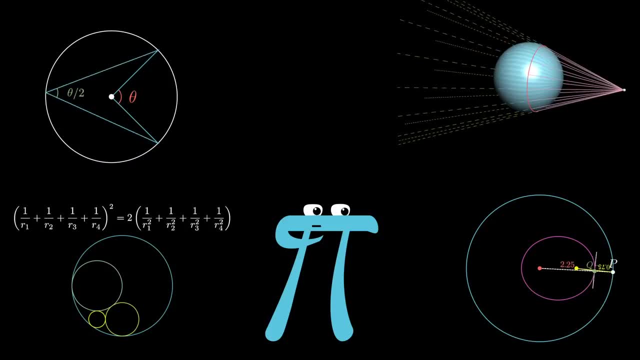 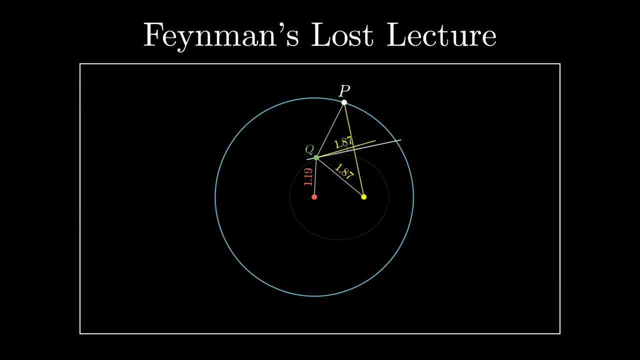 a number of other geometry problems might be particularly primed to think of adding these specific spheres. First, a common tactic in geometry is to relate one length to another And in this problem you know from the outset that being able to relate these two lengths 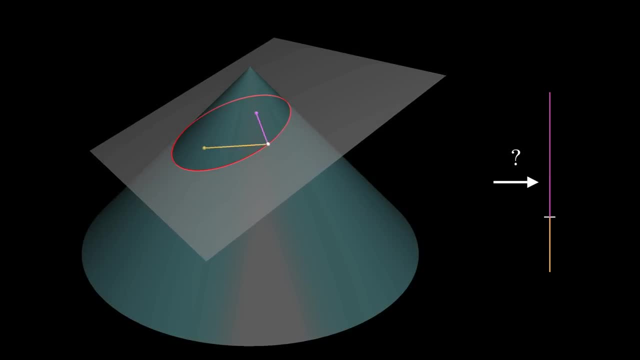 to the foci To some other two lengths, Especially ones that line up, Would be a useful thing, Even though at the start you don't even know where the focus points are, And even if it's not clear exactly how you'd do that throwing spheres into the picture. 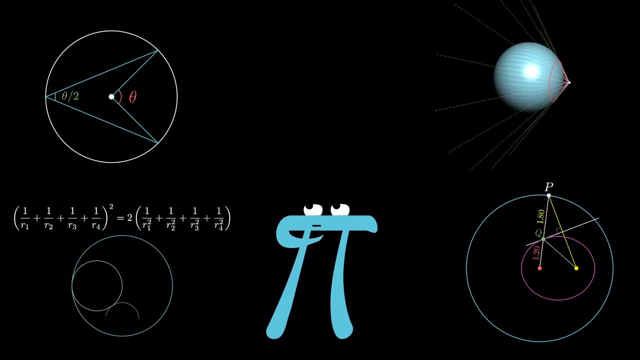 isn't all that crazy. Again, if you've built up a relationship with geometry through practice, you would be well acquainted with how relating one length to another happens all the time when circles and spheres are in the picture, because it cuts straight to the defining feature of